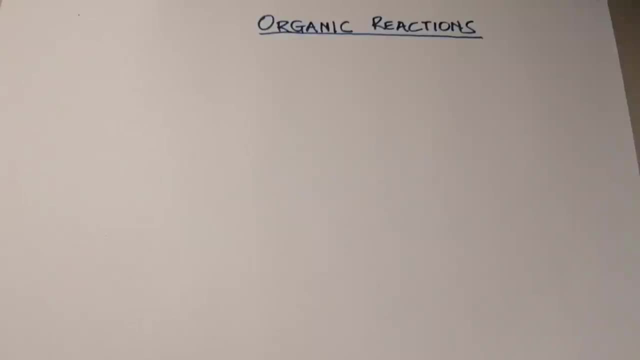 mlungesimengosi at gmailcom. All right, let's dive into it. Okay, so our first lesson. so, talking about organic reactions, So the first reaction that I want us to go through is what we call combustion. Now, they like these kind of reactions. Let's take 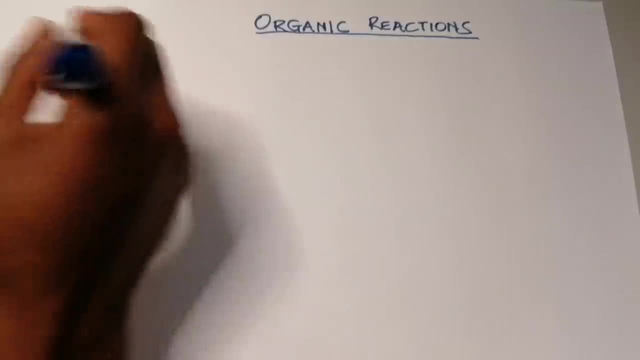 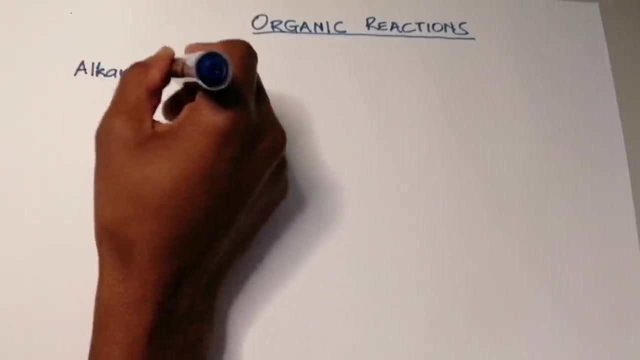 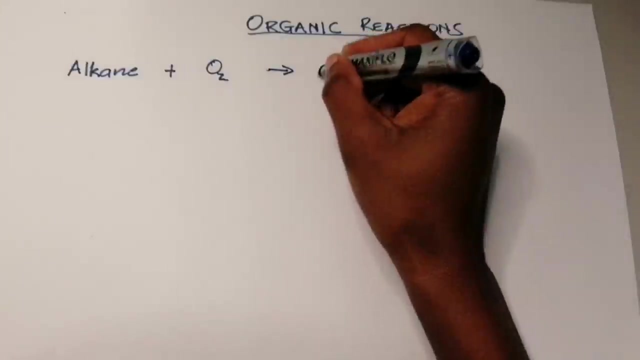 for instance, if we've got an alkane, So essentially if you take any of the hydrocarbons, so an alkane plus oxygen. So whenever you react, an alkane with oxygen, right, what you get is carbon dioxide and water, right? Just keep that in mind. 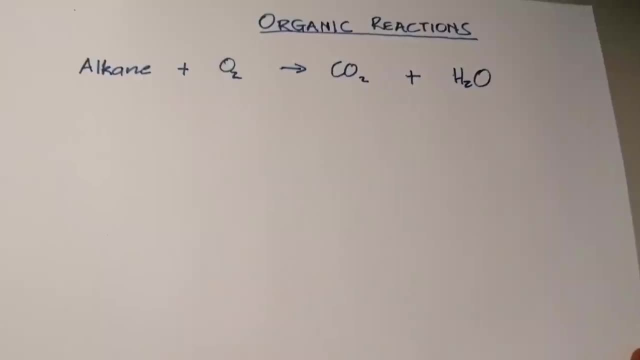 And, by the way, this is when you've got what we call a complete combustion, right? So usually it's in the presence of excess oxygen, right? If it's not in excess oxygen, so you've got what we call an incomplete combustion. 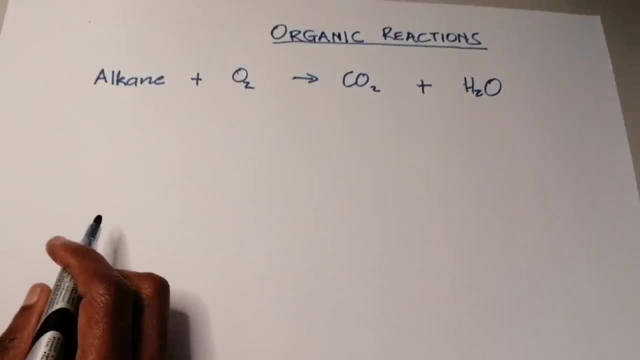 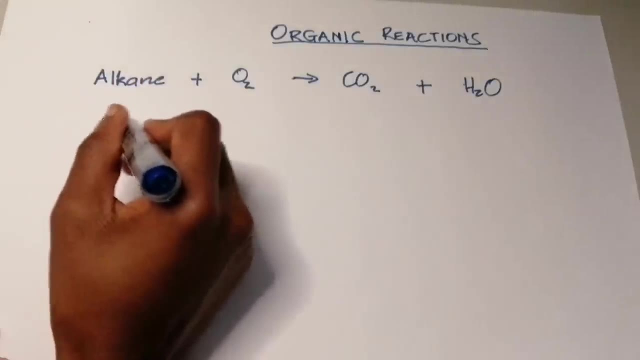 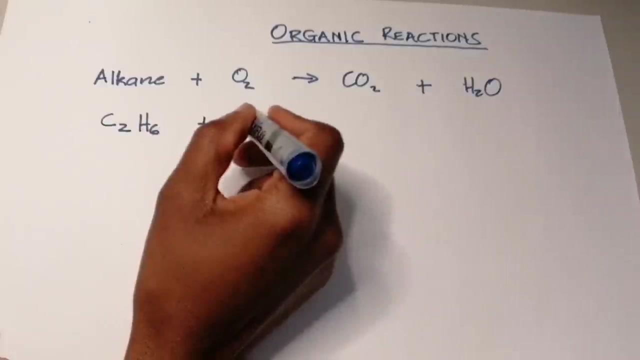 And therefore you get carbon monoxide, But nonetheless these are the most popular ones. all right, So let's take an example of that. So if we've got, say, for argument's sake, C2H6,, okay, So that would be an alkane, okay, Plus oxygen. What does it give us? It will give us. 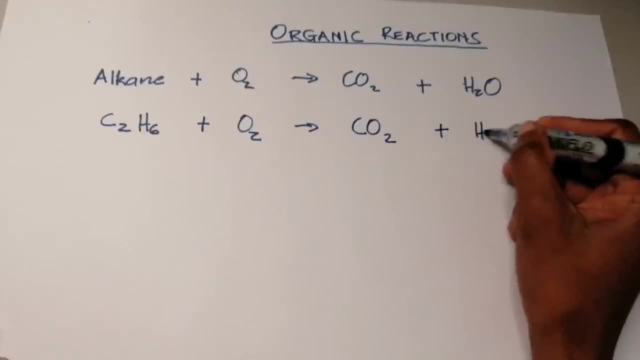 carbon dioxide, C2H6 plus H2O. Now the only thing about it is that this is not a balanced reaction. You can see that right. So now, what we want to do is now to learn how to balance them. So let's do that. 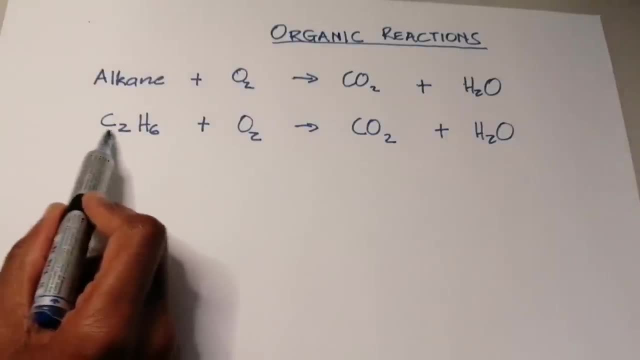 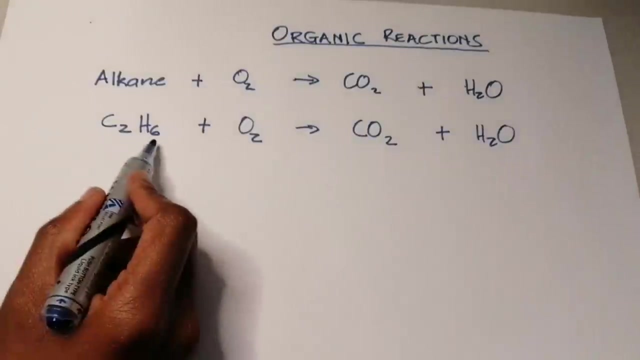 quickly. So I've got two carbons on this side. And remember, when you balance you only put coefficients right, So you don't, so that you don't change the structure of that molecule right. So in this case I've got C2H6.. So I've got two carbons on the left-hand side. How many carbons? 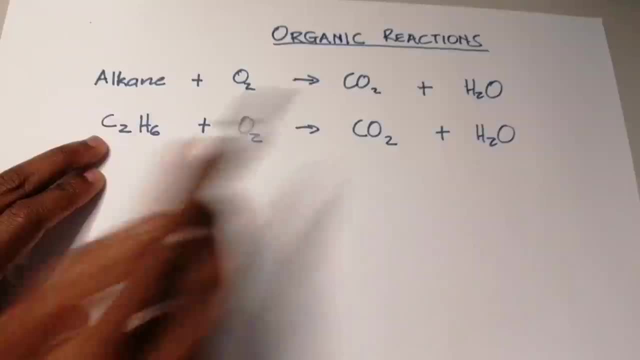 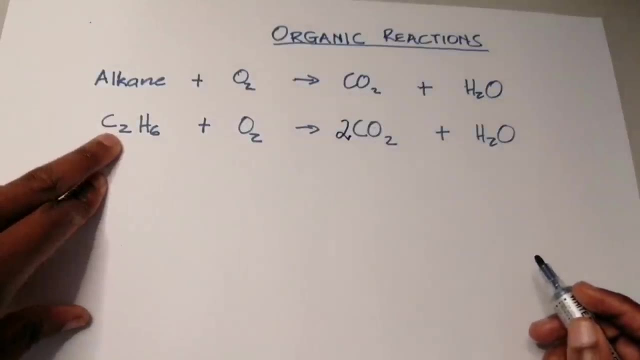 on the right. I've got one, okay. So how do I make it two? So I'm going to say, all right, so let's put a two there, okay. So two carbons on the left. okay, Now I've got two times one. 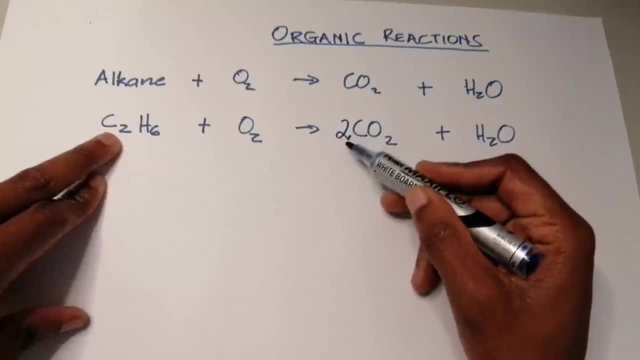 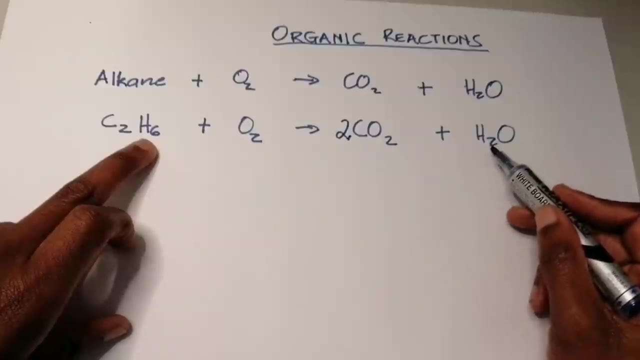 carbon on the right. So that's two carbons and two carbons. So my carbons are right. And then I've got six hydrogens on the left-hand side. Can you see that? How many do I have on the left? That's two, you're right. So in this case, how do I make the right equal to the left? Okay, 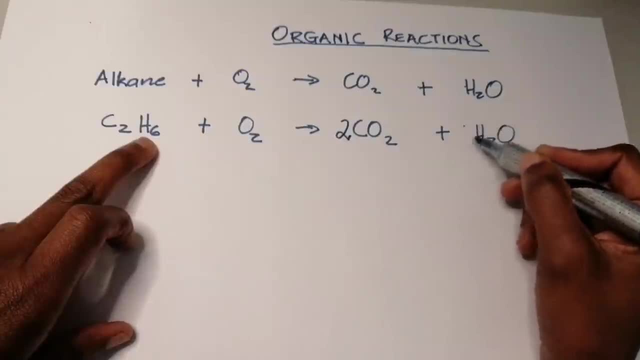 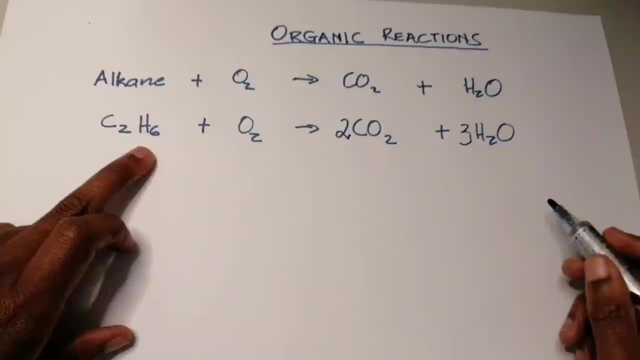 I'll just multiply that by three, because three H2s will give me six. So that's three times two, that gives me six. Okay, so my hydrogens are sorted Okay, Now what are we left with? So two? 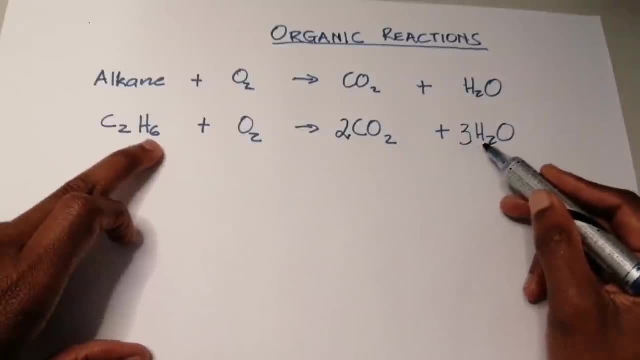 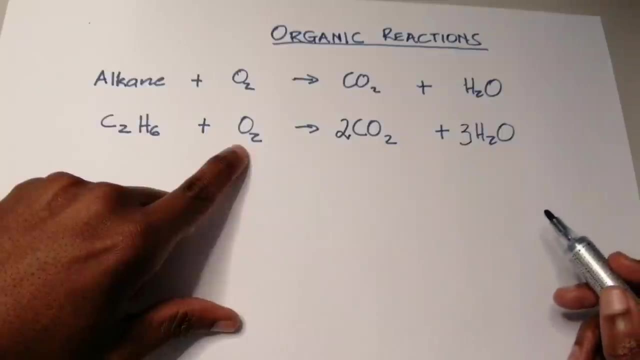 carbons. two carbons, six hydrogens: two times three is six, Okay, so that's two. So that's two H2s. So the only thing that's left now is oxygen. So two carbons on this side, okay, And then. 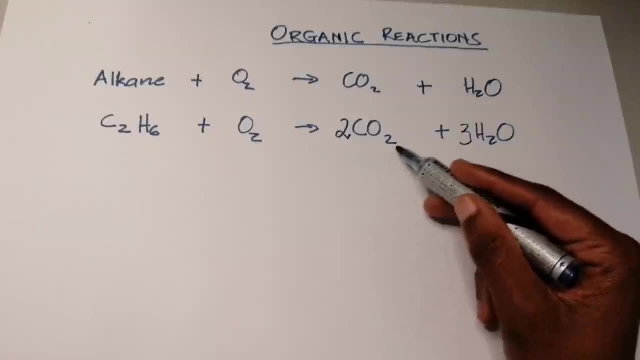 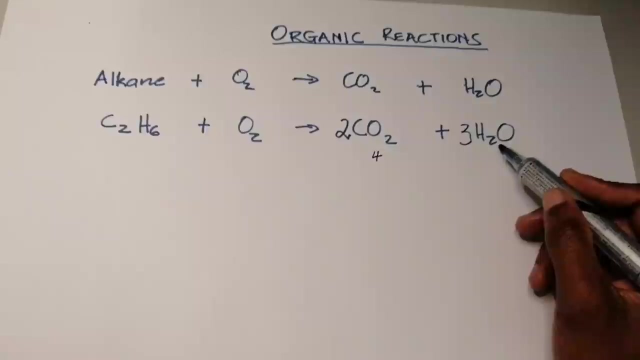 look at this: Now: you've got two times two, which is four, right? So you've got four. just on this carbon dioxide only, right? So let me just write that down there, Okay? and then you've got three times one, which is three, right? So in this case, 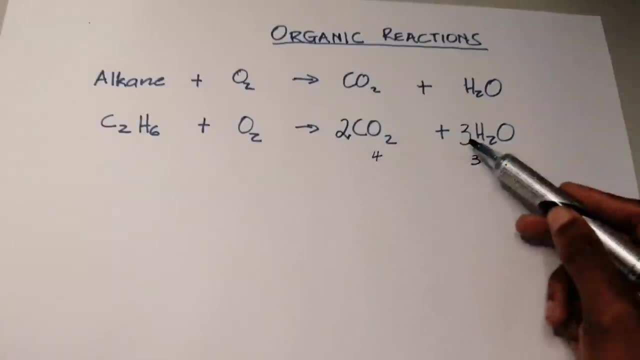 remember, if your oxygens, it's two times two, which is four, and three times one, which is three, and four plus three, that gives us seven. Okay, So now I want you to look at this On this side. 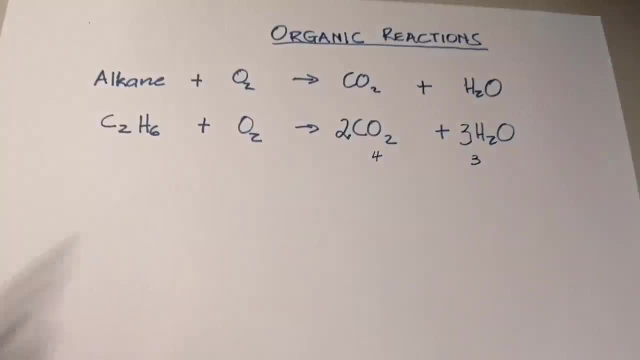 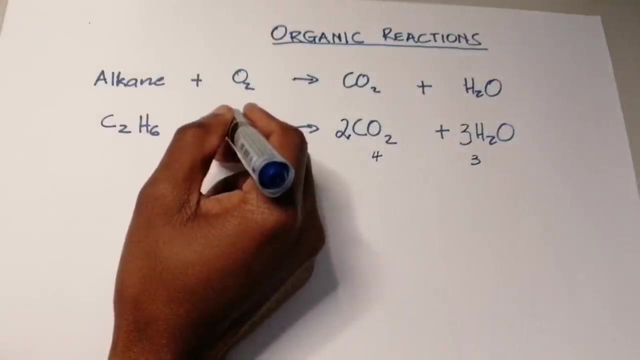 I've got two, And on that side, on the right hand side, I've got seven. So how, what do I do? Okay, so I'll simply just say: please, I want you to listen carefully- I'm just going to say: 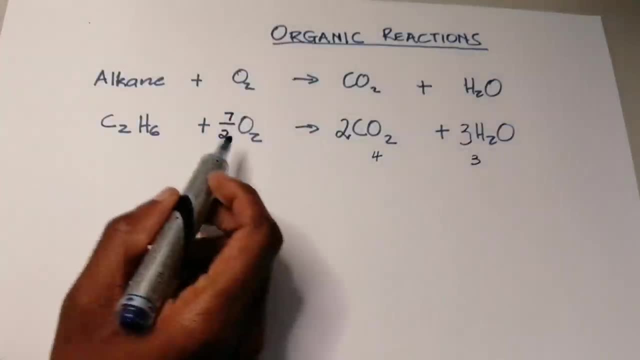 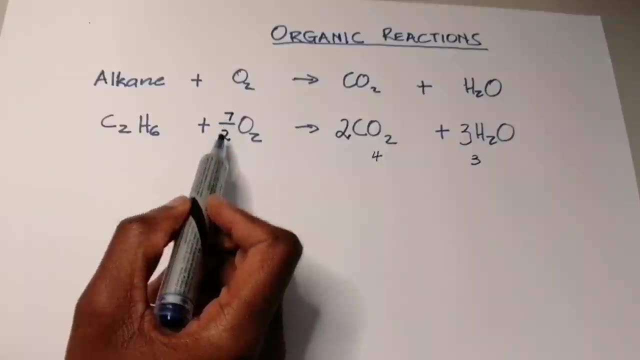 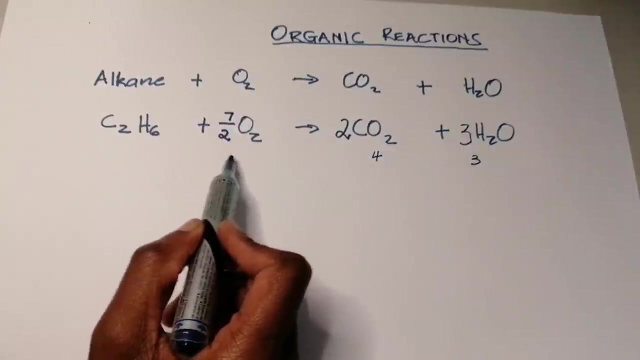 seven over two, So that's 3.5, right, Seven over two, That's going to be 3.5.. Now think about it: Seven over two times two gives me seven, isn't it? So now the number of oxygens on your left hand side is equal to the. 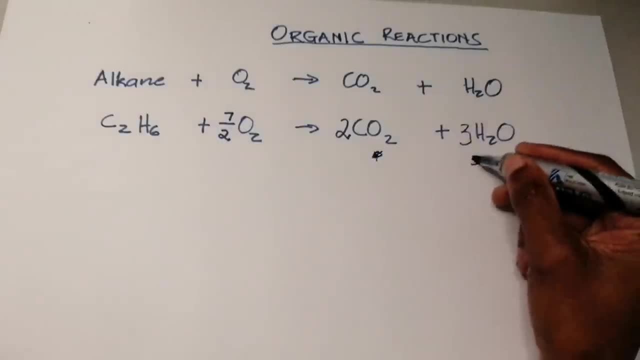 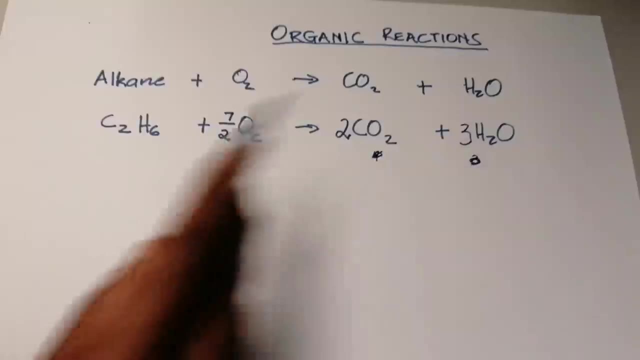 number of oxygens on your right hand side. Let me get rid of these guys. Okay, So now two carbons, two carbons, You've got six hydrogens. Three times two is six. Seven over two times two gives me seven. 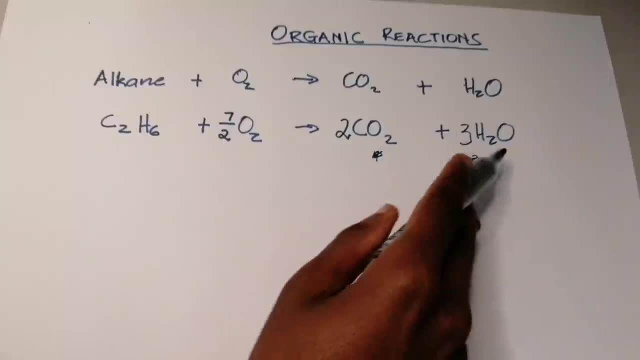 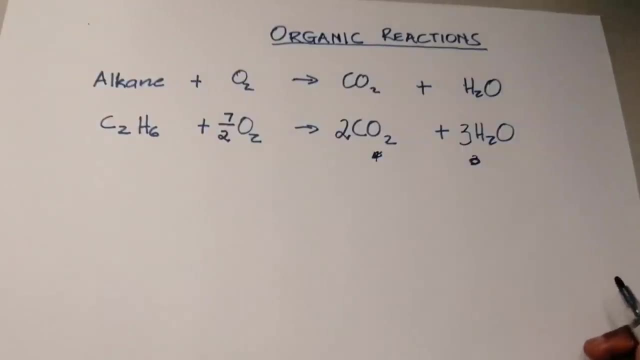 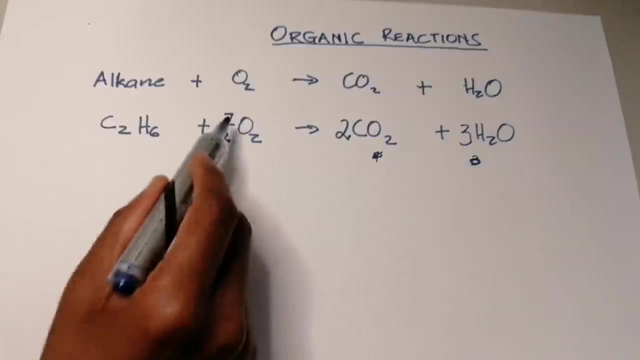 And then two times two is four, And then three times one, that's three. Four plus three gives us seven, So oxygens are complete. However, in chemistry we usually don't want our stoichiometric ratios or our coefficients or molar ratios, whatever you want to call them. 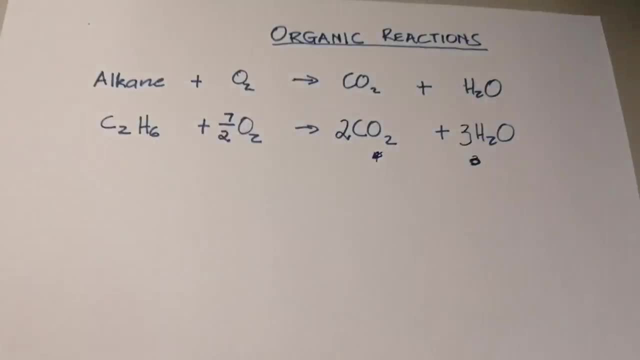 Okay, We don't want them to be in fraction form, right? Or we don't even want them to be decimals, right? So how do I adjust this? Obviously, I'll multiply in this case by the lowest common denominator. Okay, So, considering there's a one there, there's a two there, So my lowest. 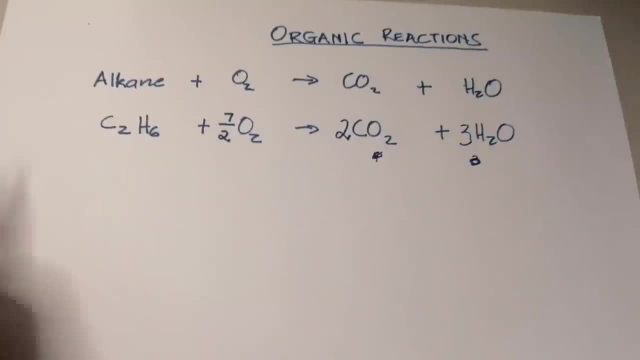 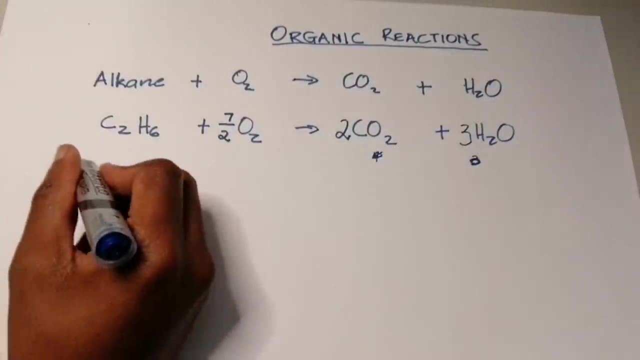 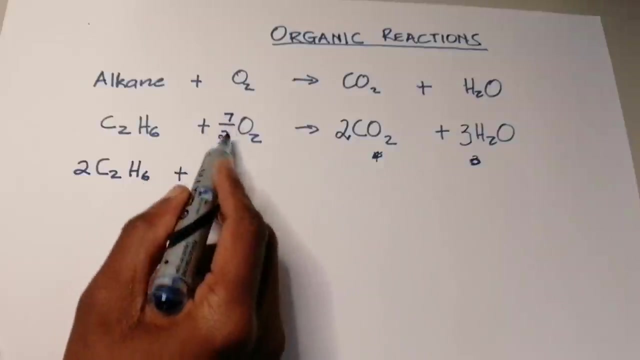 common denominator in this case is going to be two. So multiply everything by two, So what will you ultimately have? So say two times one, that's two. C2H6 plus seven over two times two, So that's seven over two times two. Remember we said we're multiplying everything by two, So seven over two. 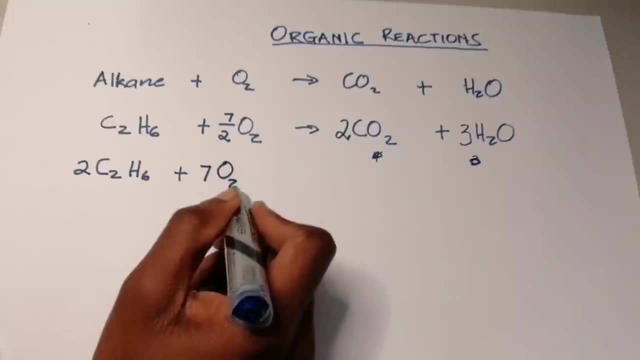 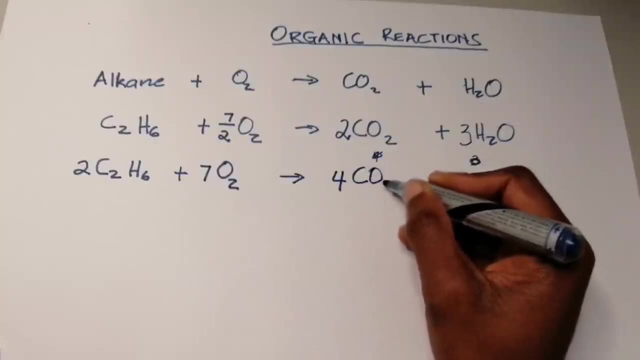 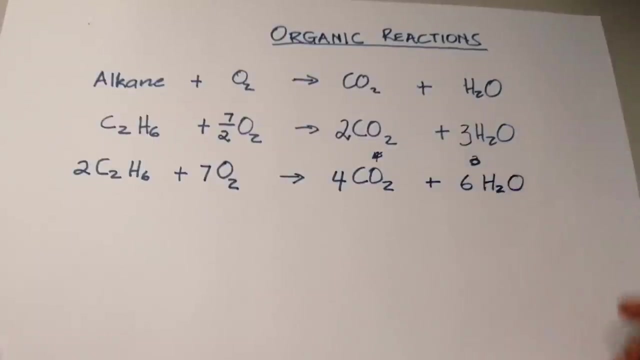 times two, that gives us seven, So that's seven over two. And then what does that give us? Two times two, that's four. Okay, So that's four. carbon dioxide plus three times two gives me six, So that's six H2O- Okay, So that's a combustion reaction- Okay. So that's how you would do that. 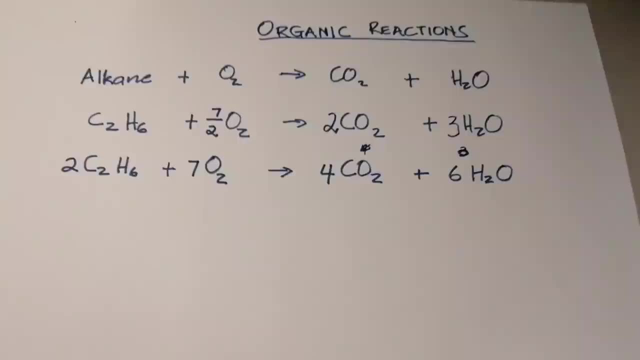 By the way, you can check out my website at wwwh2ocom And I'll see you in the next video. Bye, do this with alkenes. You can do that with alkynes, Just remember, Okay, Perhaps, maybe we. 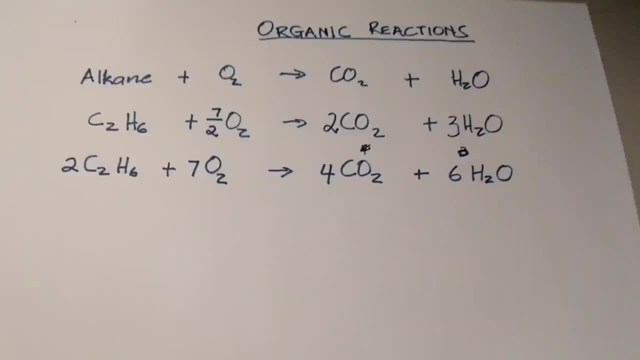 want to take just another example so that you get the gist of it. Okay, Right, So, okay, let's take something else. Let's say we are going to take C3H8.. Right, Okay, So let's say C3H8.. Okay. 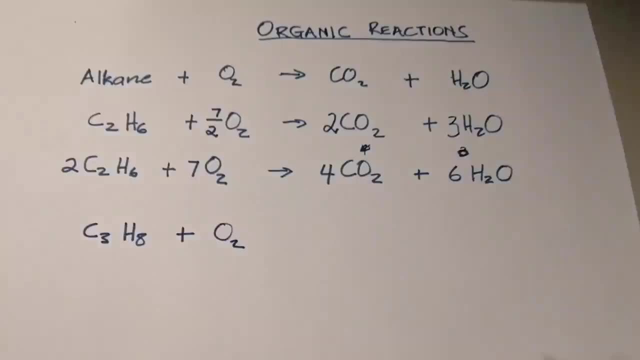 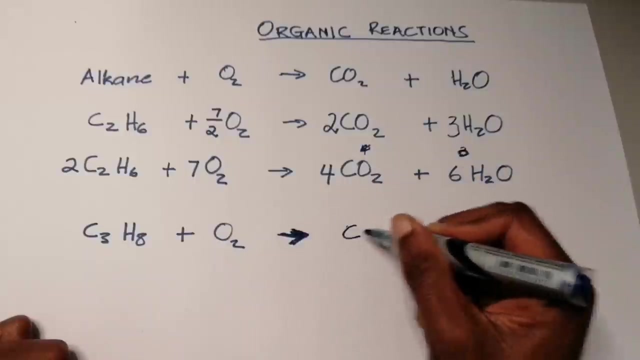 So plus oxygen, So that's a complete combustion, isn't it? So we're going to say: right, so you already know, sorry, what the products are, isn't it? So our products are going to be carbon dioxide, Sorry about that. So our products are going to be carbon dioxide. 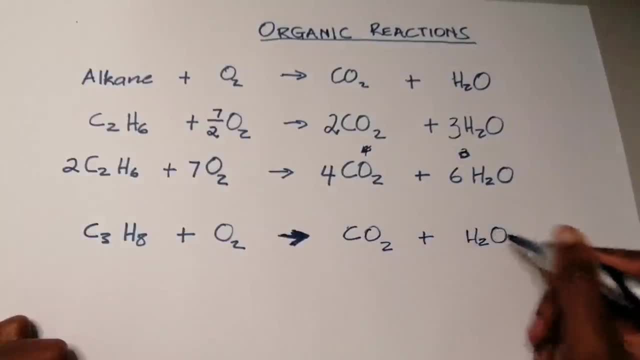 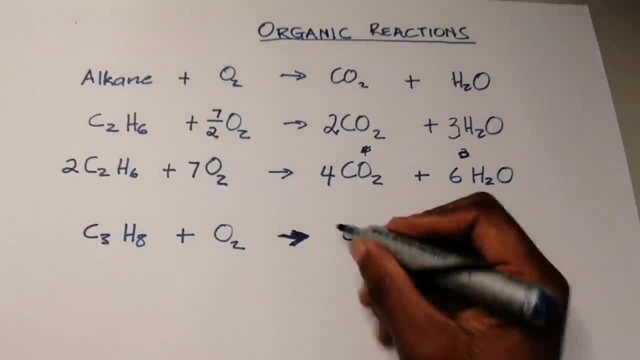 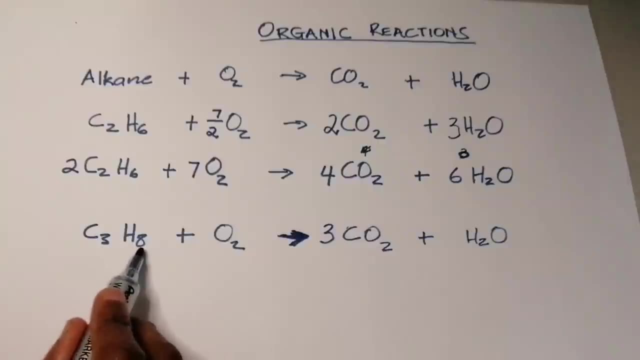 we have C3H8.. Got only one carbon there. So what do you do? Just simply multiply that by three. So three times one, that's three, That's three carbons, And then eight hydrogens. Okay, So you're. 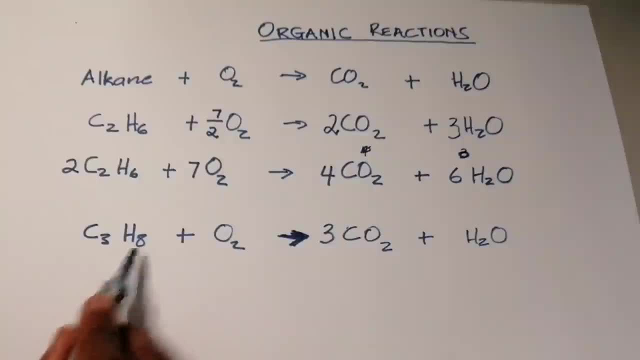 going to say: okay, so the number of hydrogens, that's eight, Right. And how many do you have on the right hand side? You've got two hydrogens, Right. So how do you make it eight? You just simply multiply that by four. Okay, Right. And then so: 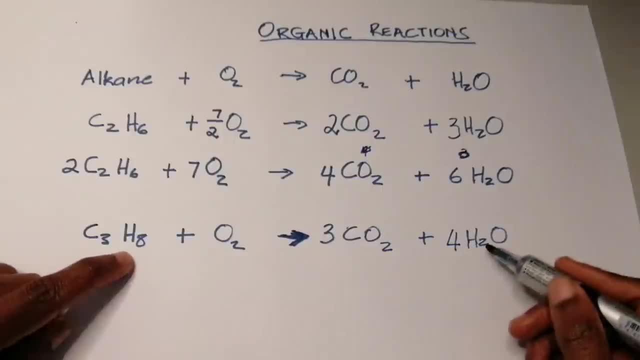 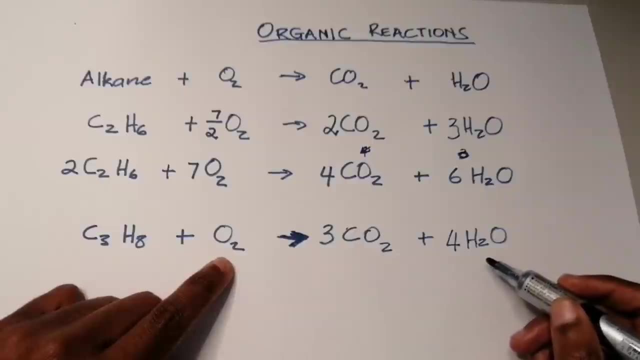 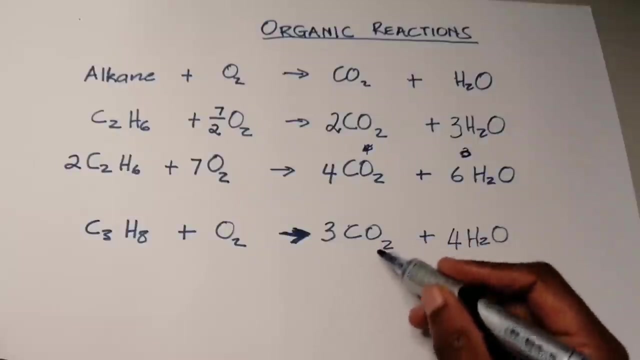 three carbons, three carbons, eight hydrogens. four times two is eight. So that should be fine Now. what we're left with now is the oxygen right. So we've got two on the left hand side And then three times two. that's going to be six. And then you've got four times one. 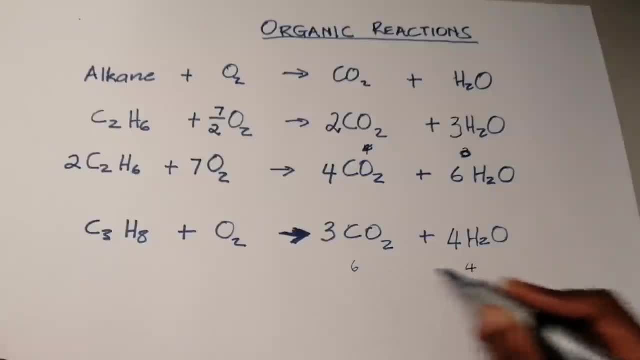 which is four. Okay. And then six plus four gives me 10, right? So in this case you've got 10 oxygens on the right hand side. How many do you have on the left hand side? You've got two. How do you make that 10? You just simply multiply that by five. Okay, See. 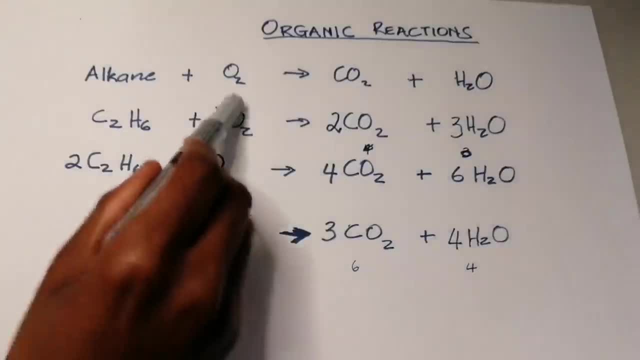 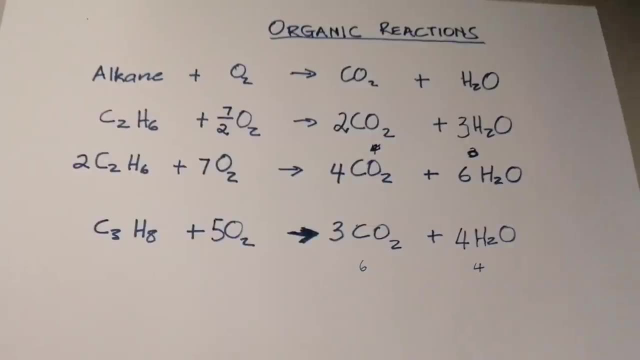 this one was easier because you didn't have the previous situation where you had one of them being a fraction, right? So now what you want to do is maybe just try, try one on your own and just see my solution thereafter. right, Okay, Maybe let's just take. 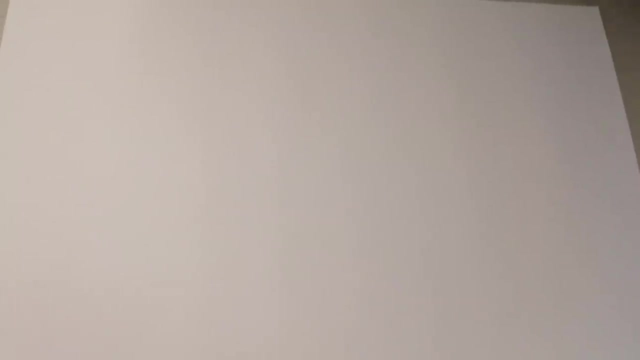 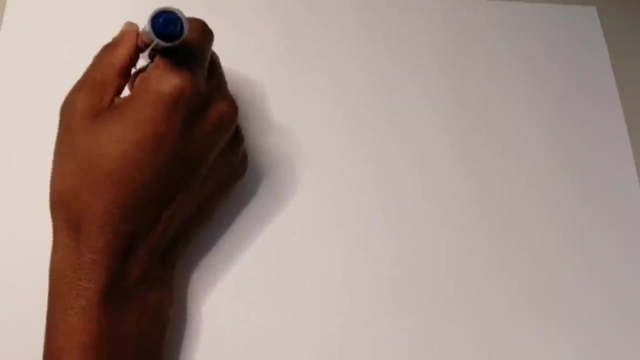 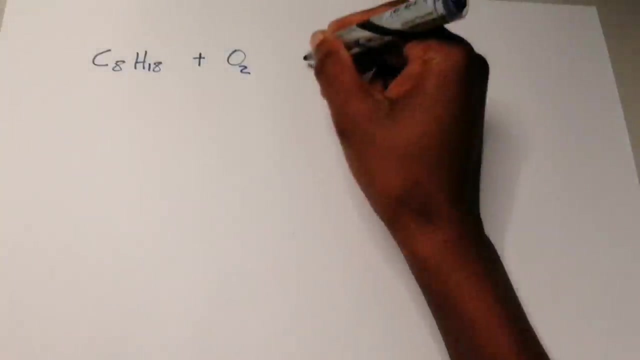 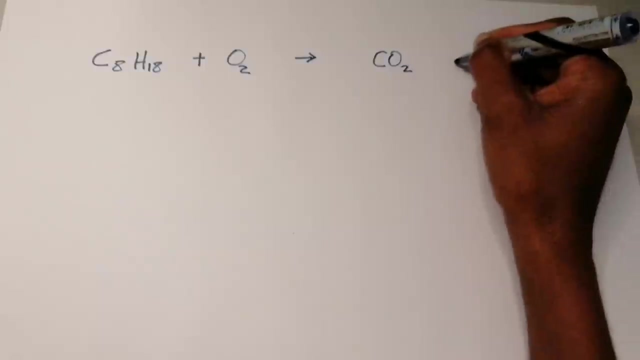 another page. Okay, So suppose we take. yeah, let's take petrol, right, So that's C8H18 plus oxygen. By the way, this is the reaction that happens inside the engine of a car: That's going to give us carbon dioxide. that comes out the exhaust, By the way. 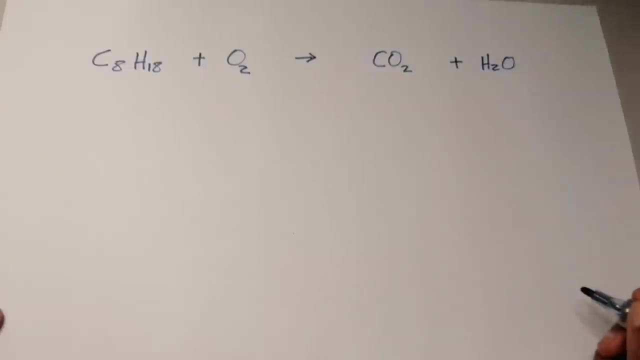 these combustion reactions are exothermic, And what we mean by that is that they always release energy. Okay, So energy is released in the process. Okay, So they're always exothermic. or you can just simply express it as: delta H is less than zero. Okay, So these are always. 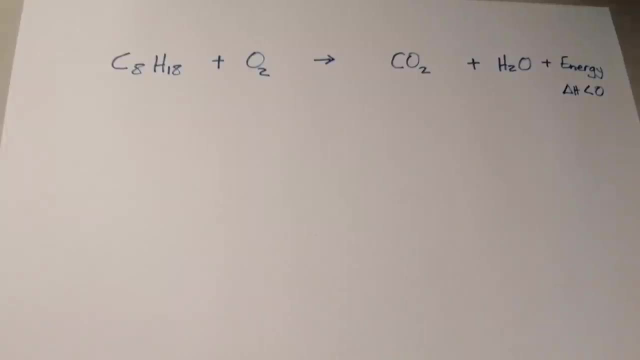 exothermic reactions. So you can just simply express it as: delta H is less than zero. Okay, So these are always exothermic reactions. So please try that on your own, And then afterwards you can just put the solution for me at the bottom as your comment. Okay, Right, I just want to see. 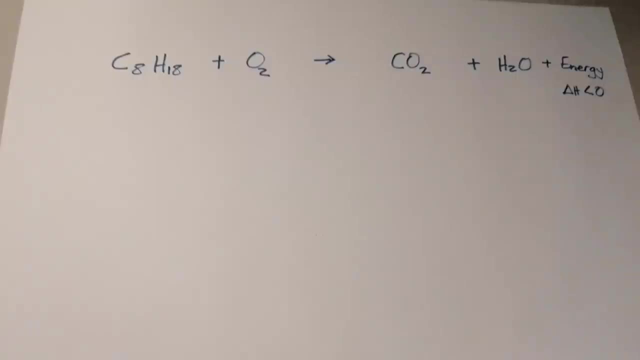 if you guys get it Right. So now I want us to move on to something else. Okay, I'm going to move that away. So I want us to move to other reactions in organic chemistry. Now, um, another reaction that we have. 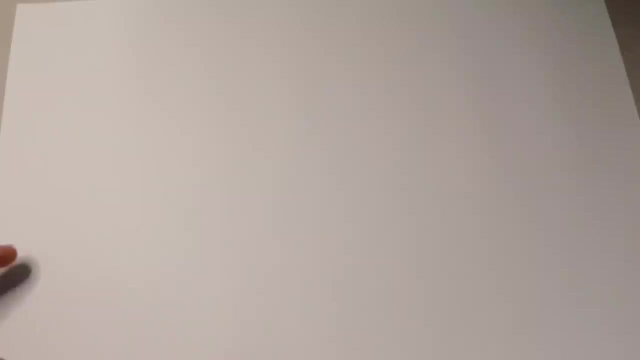 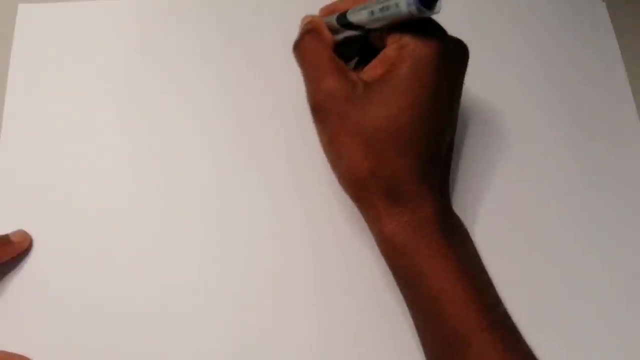 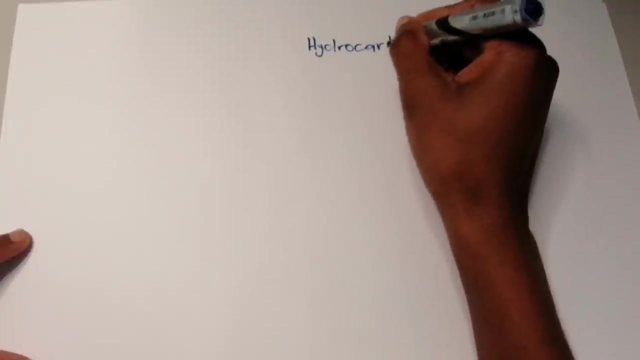 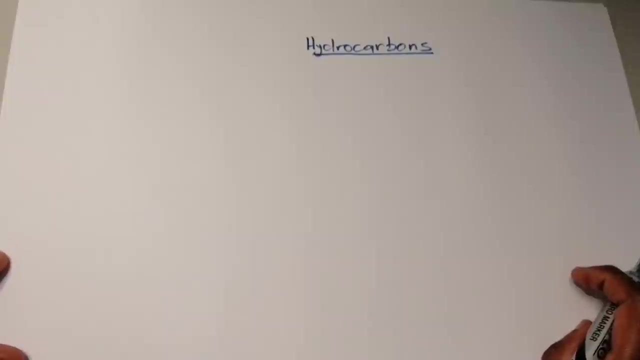 two types of substances that we have okay in organic chemistry. So we've got what we call Okay. So when we take our hydrocarbons, um so hydrocarbons carbons, Okay. So we've got alkanes, alkenes and alkynes. But now, uh, with your hydrocarbons, you've got two types. 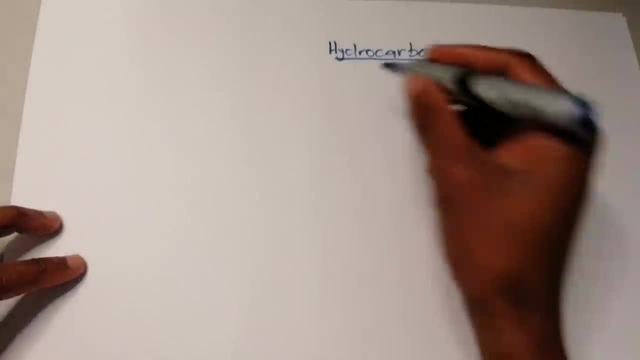 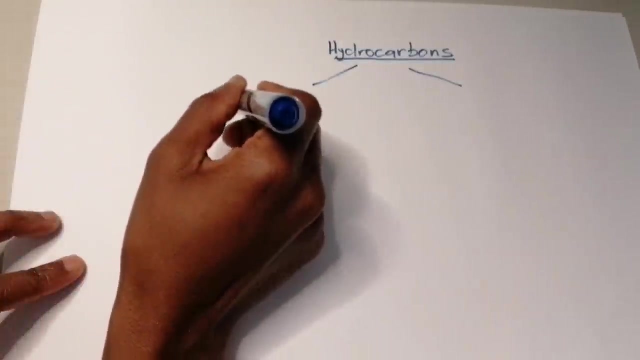 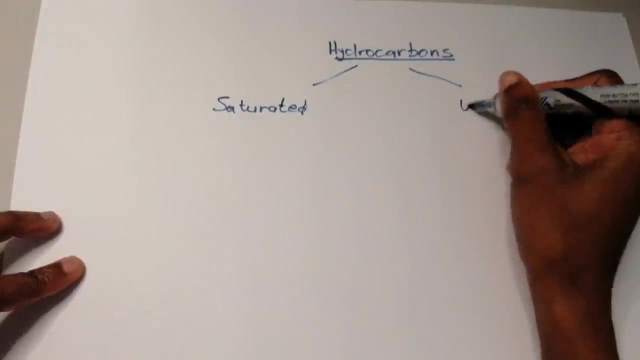 um type of reactions, Okay, Or uh, you know you've got. you know you've got, you know you've got two types of compounds that you have. We have what we call saturated hydrocarbons- Okay, Saturated- And we've got what we call unsaturated. Now, with our saturated unsaturated, 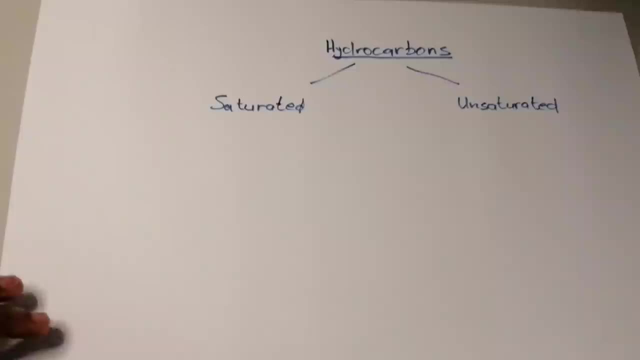 Okay, So with our saturated hydrocarbons? uh, those are the alkanes, So those are the ones that are only between uh adjacent carbon, uh, um, uh, uh, atoms, right? So in this case, 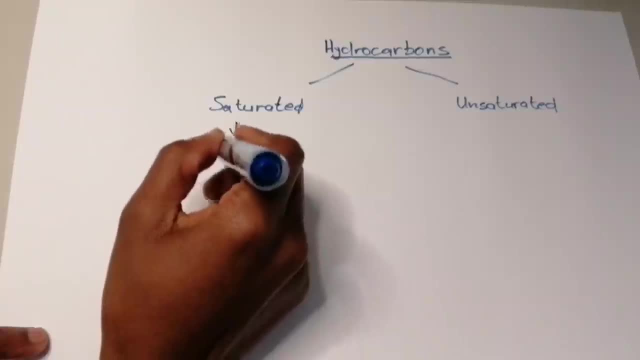 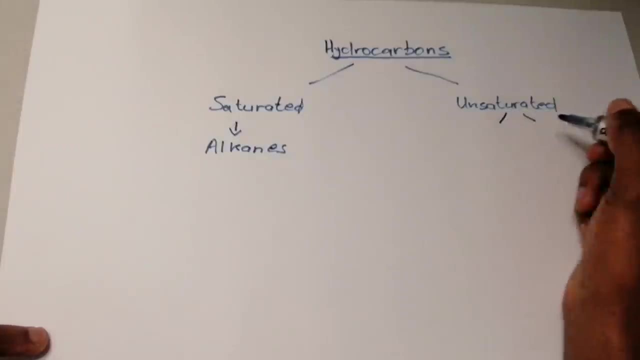 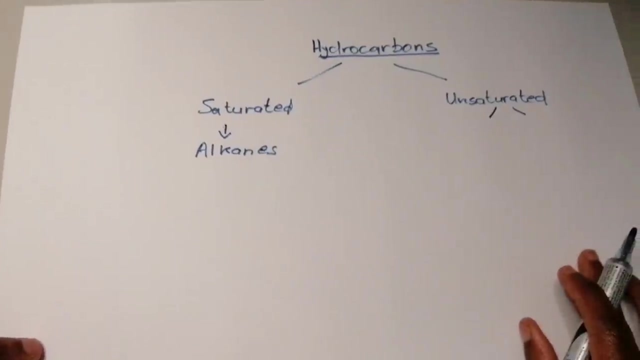 you've got saturated, which are your alkanes- Okay, And then under unsaturated, they either have a double bond or a triple bond. Remember, we are talking about hydrocarbons, right? So that can only mean that we are referring to um alkenes. 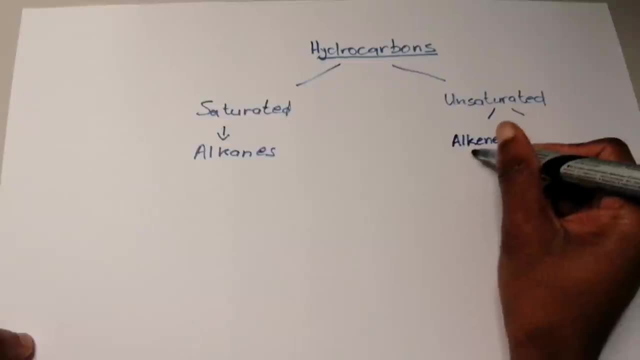 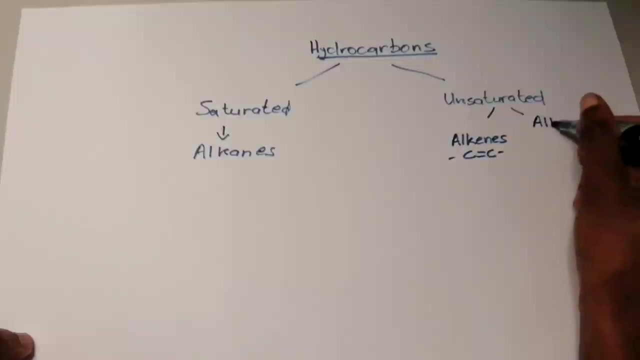 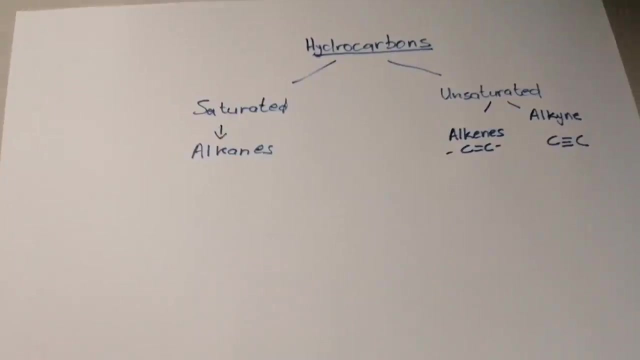 All right. So the ones with the double bond, okay, And between carbons, or you're talking about alkenes. Okay, And alkenes, obviously the ones with a triple bond between adjacent carbon atoms, right. So now type of reactions that uh occur, uh, on those we say well, 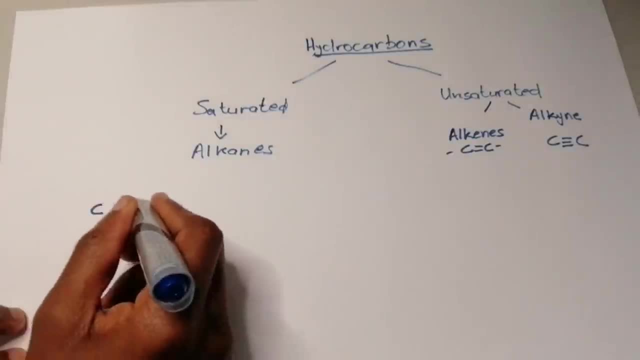 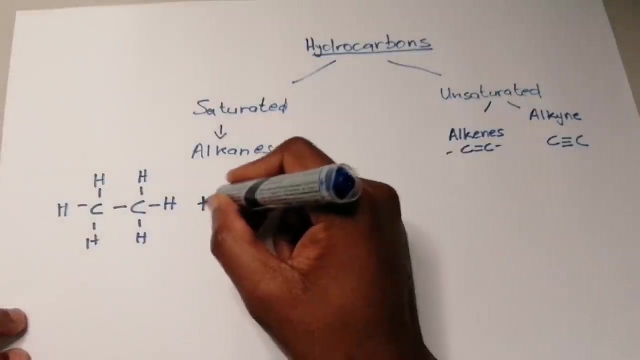 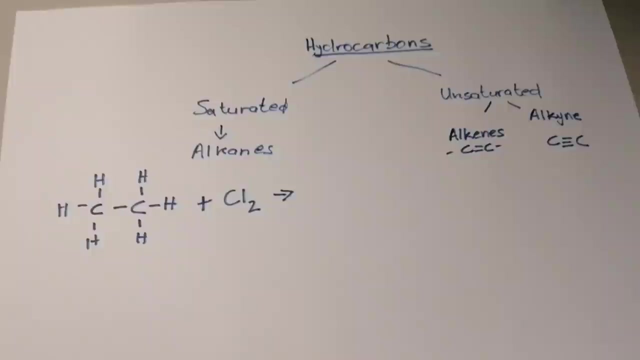 suppose that we've got an alkane and it reacts. Okay, So let's take a simple alkane and we're going to cause it now to react with a halogen. Okay, So let's take a simple halogen again. So we say: well, if we take an alkane and it reacts, 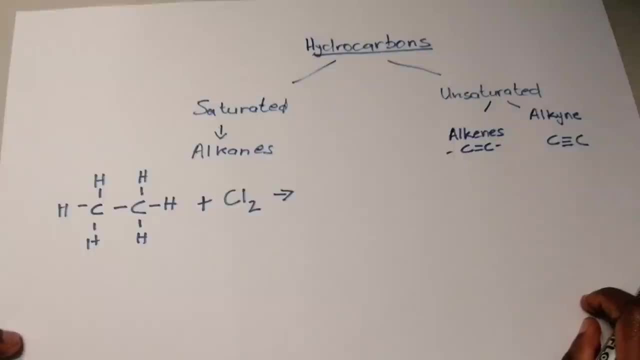 with a halogen. what type of reaction takes place there, right? First of all, um, I want you to know that those reactions usually don't occur unless we do something else, And that is, we put in, uh, UV energy. Okay, So it means that? 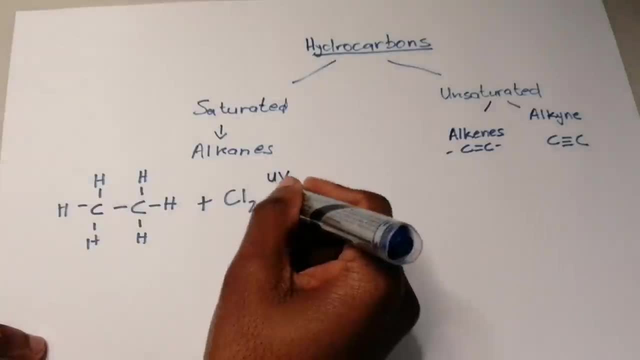 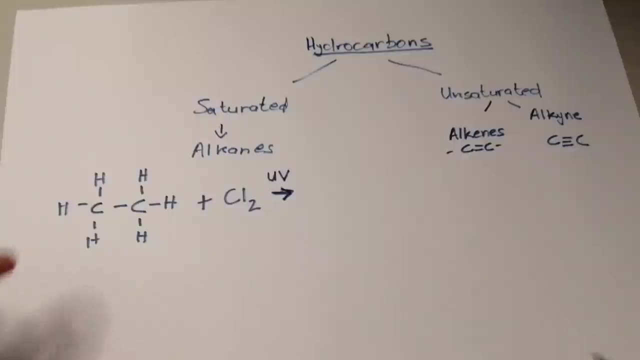 they are non-spontaneous reactions. Okay, So these are reactions that will not be able to take care. I mean, uh, take place on their own right. So therefore, when you put in UV energy, you force the reaction to occur. Okay, So that's the reaction that will not. be able to take care. I mean, uh, take place on their own right. So, therefore, when you put in UV energy, you force the reaction to occur, Right? So therefore, when you put in UV energy, you force the reaction to occur. 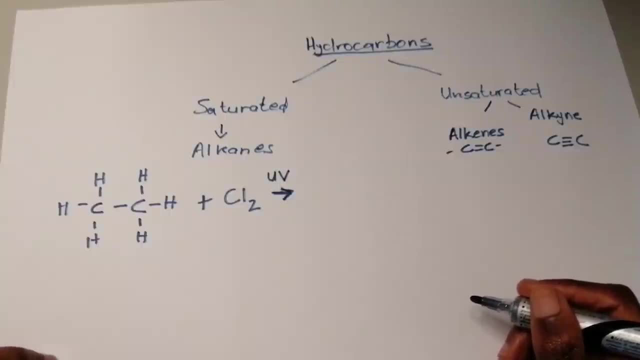 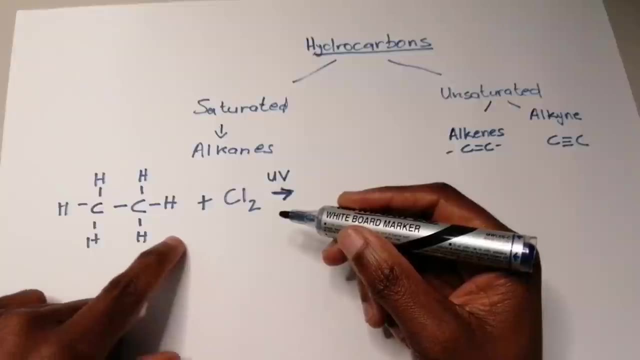 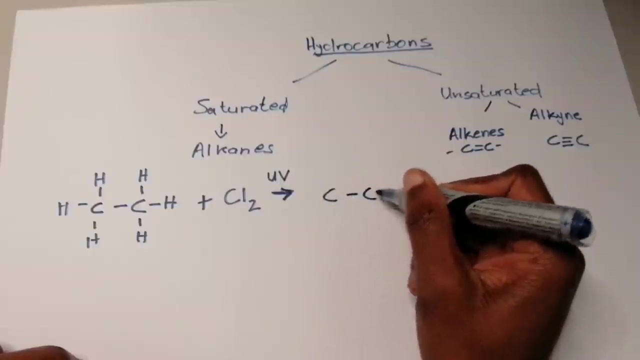 Uh, but otherwise there wouldn't have been a reaction that takes place. So what type of reaction occurs there? Right? So one of the chlorine atoms will now go and substitute one of your hydrogen atoms, right there, right? So what you end up with, I want? 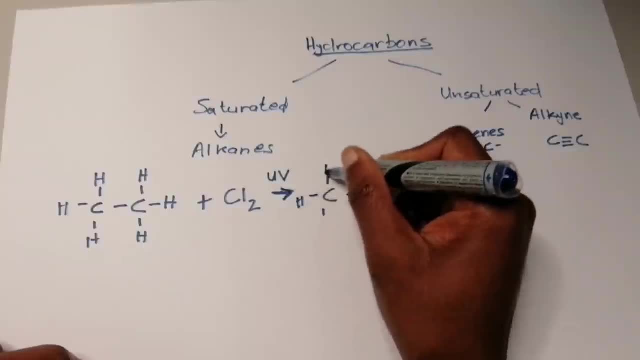 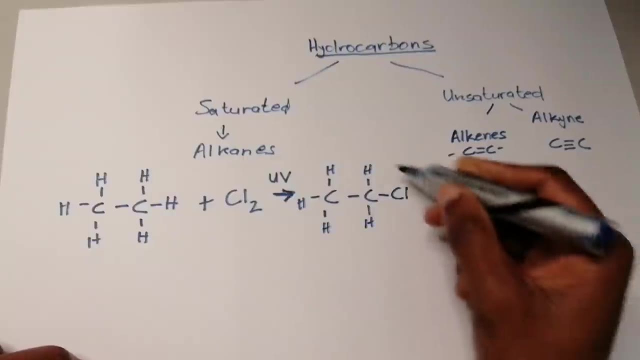 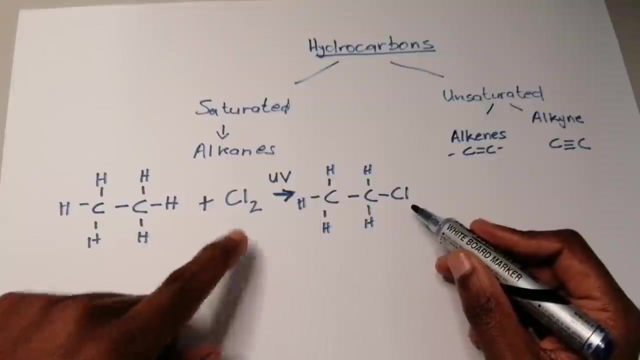 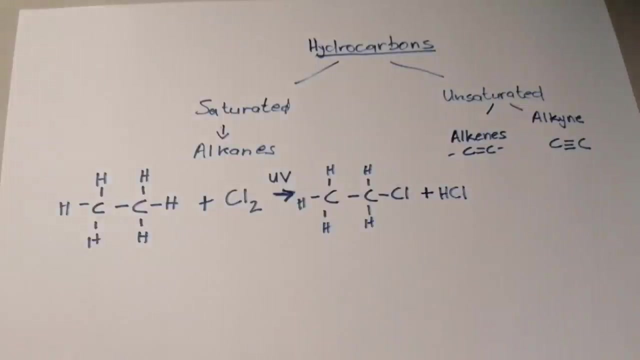 you to please note. So we end up with something like this. Okay, and please keep in mind, right, so you end up with something like that. but now remember, you still have a chlorine atom there and with the hydrogen that came off. so this is plus hcl. okay, right, and now we call these type. 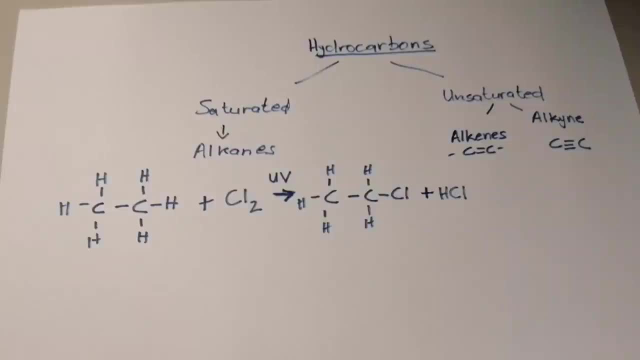 of reactions we say these are um substitution reaction. this is a substitution reaction, okay, so saturated hydrocarbons will tend to undergo substitution reaction. so in this case we call this type of reaction a substitution reaction. substitution- okay, for obvious reasons. right, one came off and was replaced by another, okay, so these are the type of reactions that tend to. 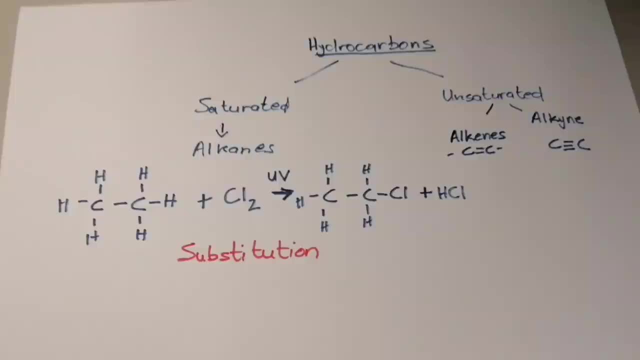 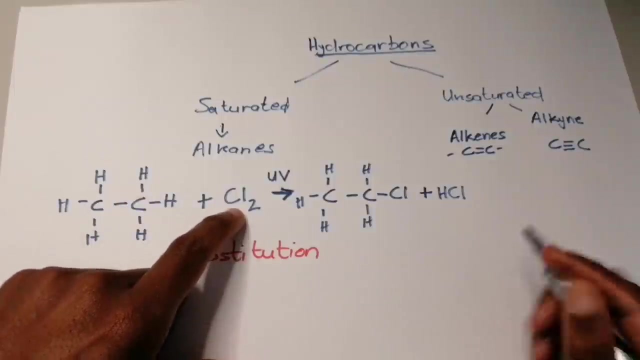 take place in alkanes. all right, by the way they can. they can also ask what type of substitution reaction. this is okay. so what did we react with? we took an alkane and we reacted it with an- a halogen. okay. so this would be halogenation. so this would be a halogenation reaction, okay, um, by the way, there's 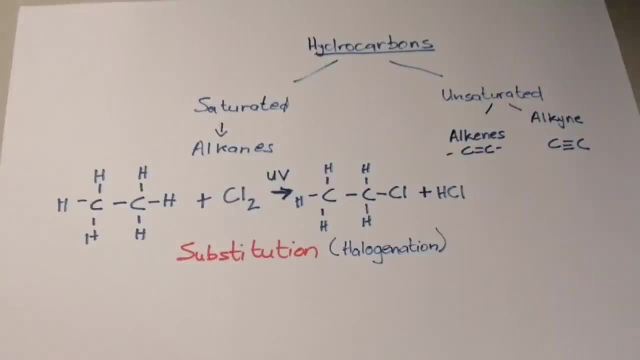 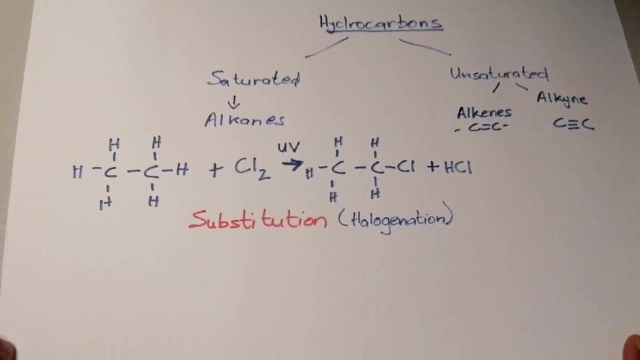 nothing wrong if you wanted to say chloroform. chloroform, okay, because specifically this time, the type of halogen that we used was chlorine, right? and then, uh, what happens when we take any of those? let's take an alkene, right? so what type of reactions do unsaturated hydrocarbons undergo? so let's take another. 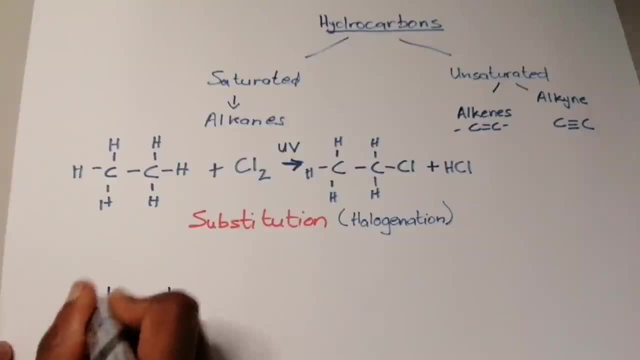 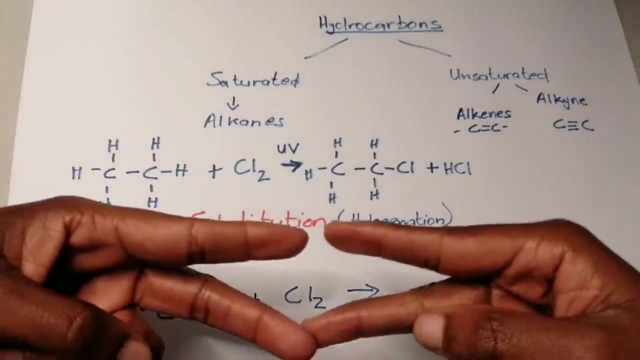 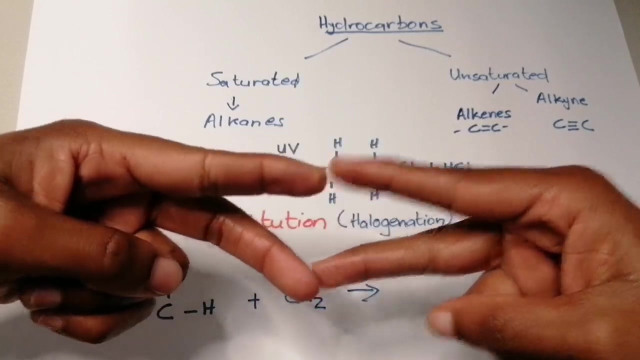 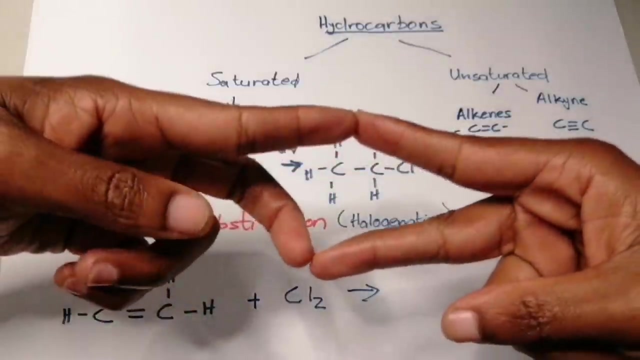 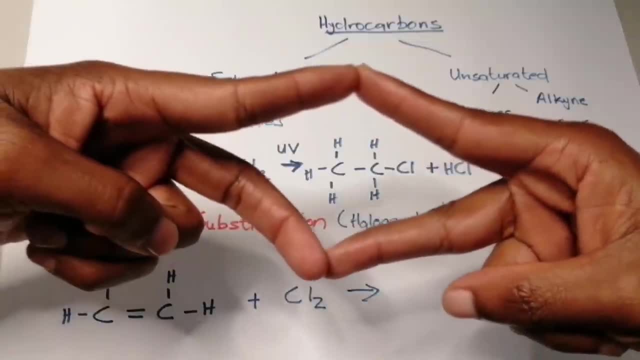 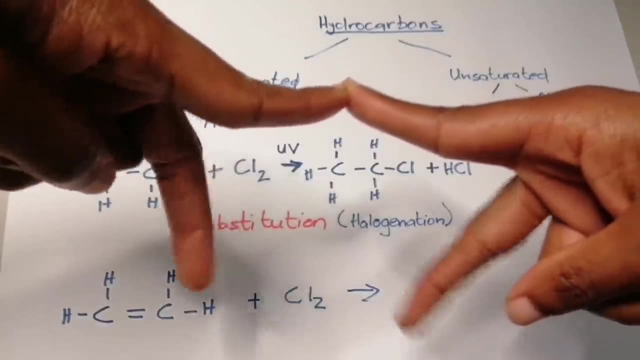 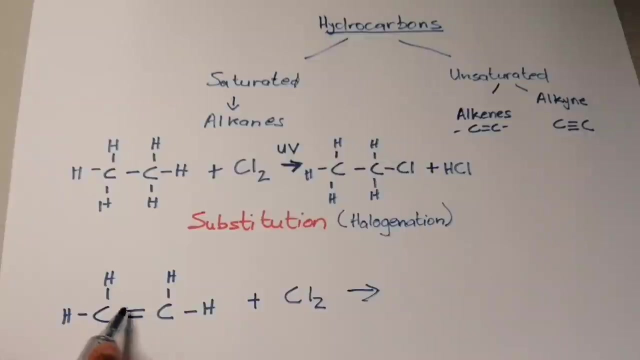 which is a weaker one, so it's this one here, okay? so when it breaks, okay, i want you to see. so when it breaks, now i've got two fingers that can basically hold to hold on to something else, right? so, um, when a double bond breaks, now, here it is. we've got the sigma bond there and we've got the pi bond. okay, right, not that you need to know their names, right? so what happens? so now, uh, by the way, these tend to 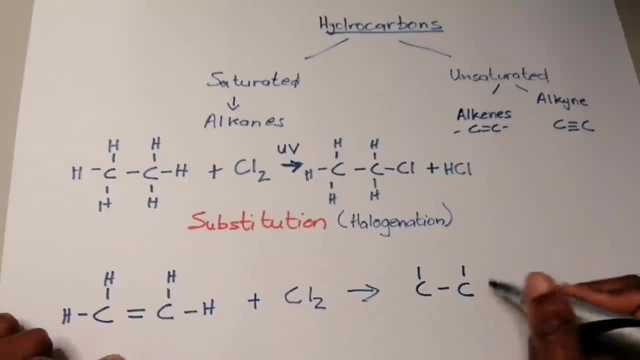 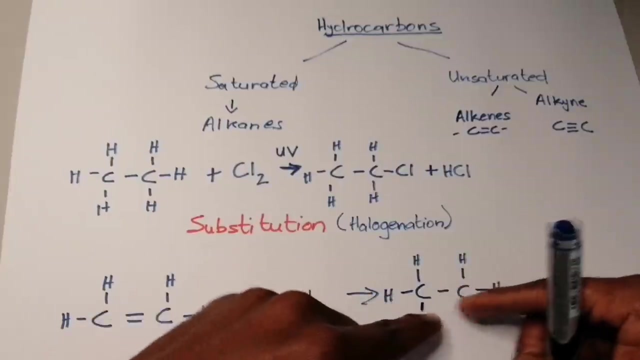 okay, more spontaneously, okay, so, uh, in this case we say all right, so this is what we have. so, note: we broke the double bond, okay, and now we've got um two arms or two hands that are available there, right, remember, those are the ones that form the second bond. okay, so those are the two. 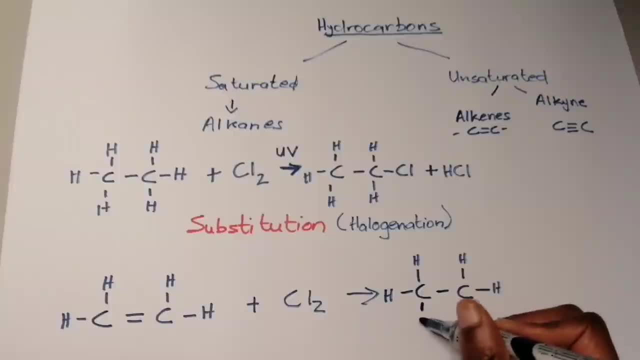 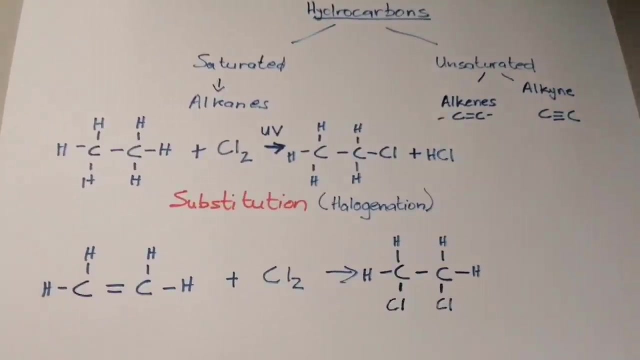 um vacancies, if you want to call them that. right now, what happens? this chlorine? the first atom comes there, okay, and the second one goes there, all right. now we say unsaturated hydrocarbons undergo what we call in this case a an addition reaction. so this would be addition reaction. 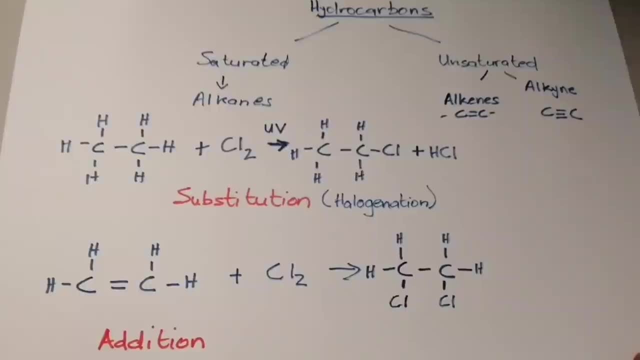 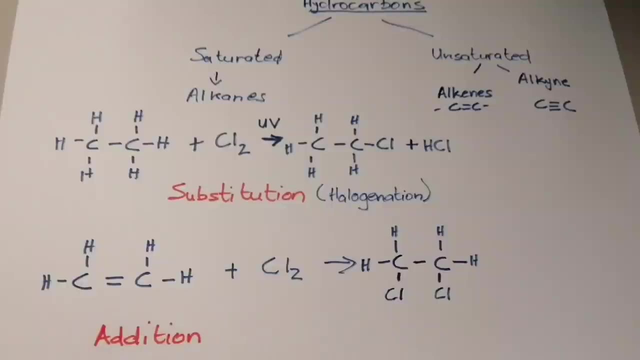 okay, right, and by the way, what type of addition reaction is it again? um, funny enough, it has exactly the same name. you are adding chlorine, so obviously, again, it would be halogenation. okay, halogenation, and in particular, by the way, uh, it is chlorination, okay. 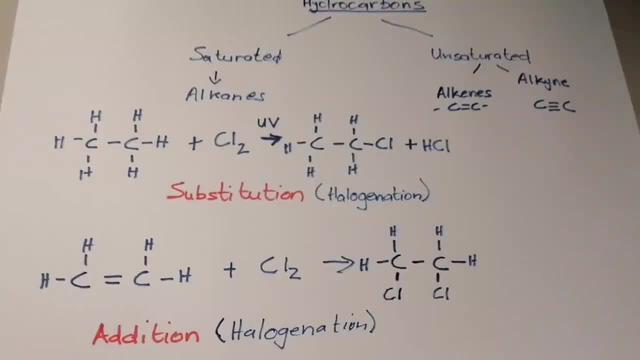 so these are the type of reactions that, um, alkanes or alkenes tend to undergo. so you must just note: okay, so alkanes, when they react with halogens, okay, they will undergo substitution reaction. and, by the way, please just note that we've got a byproduct and then alkenes undergo an addition. 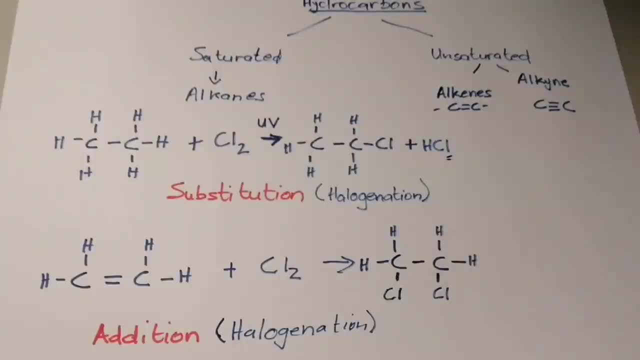 reaction and in this case, there was nothing, um, that was formed there, okay, uh, just to remind you, okay? so what would we name that? okay, this would be 1,2 dichloroethane. can you see? so we moved it from being unsaturated now to being saturated. okay, so that's another. 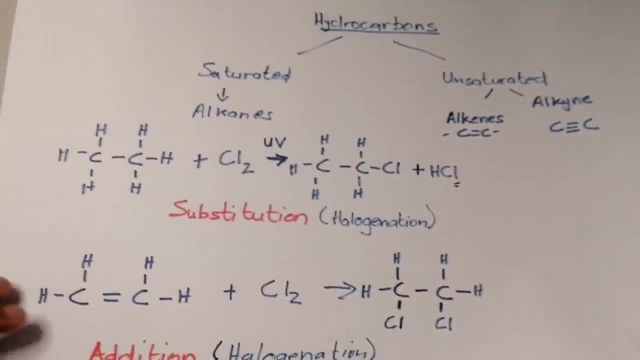 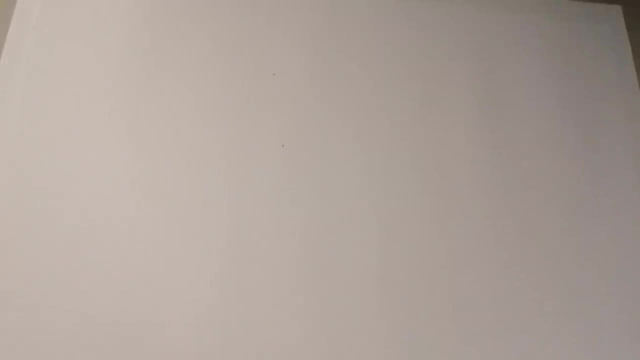 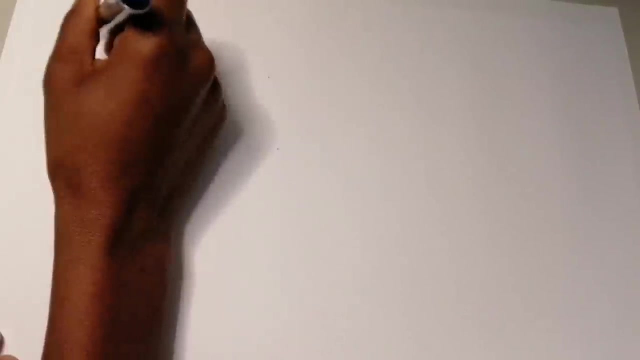 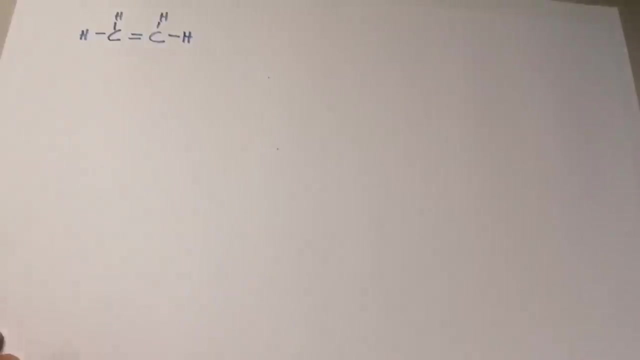 addition reaction. by the way, um, there are other types of addition reactions that may occur, right? uh, let me just show you those quickly, okay, so, um, what are the other addition reactions, uh, that we can have? okay, so, we can have a situation where we take an unsaturated hydrocarbon, okay, um, all right, let's take that ethane. 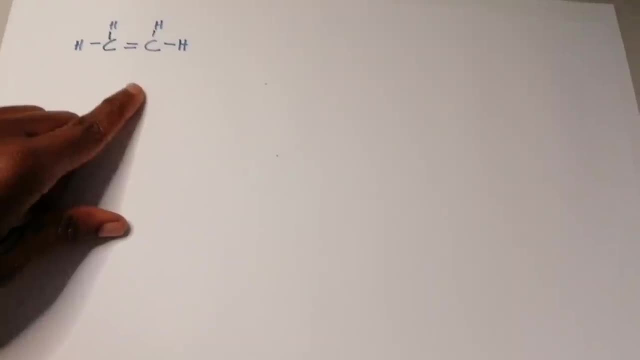 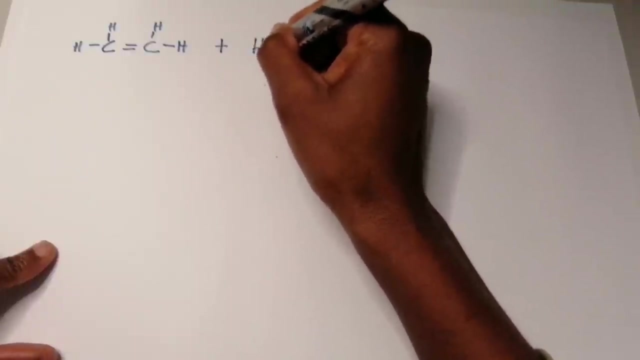 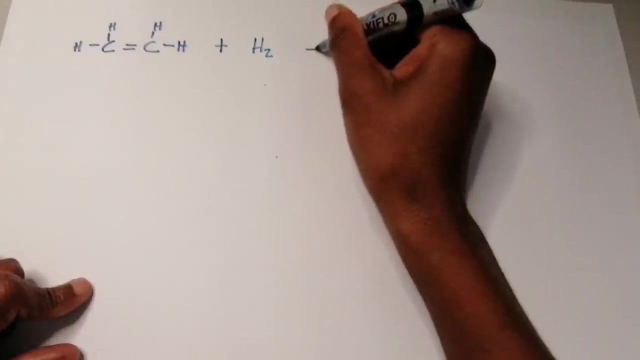 sorry, ethene again. right, so it undergoes a reaction, right. so now let me react it with hydrogen. okay. so what am i doing? i'm moving it from being unsaturated to being saturated, okay. so what happens? that double bond breaks there. the second bond, the pi bond. 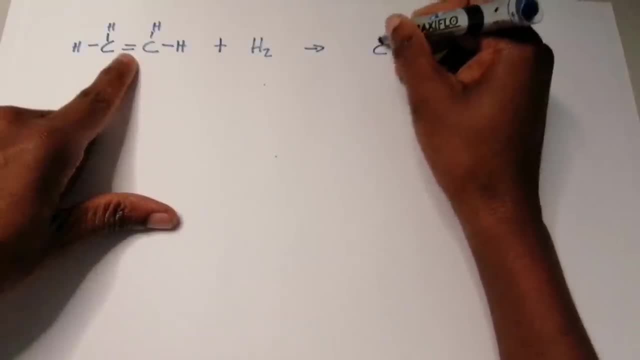 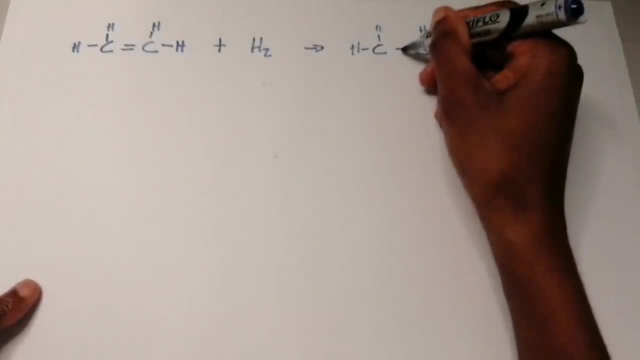 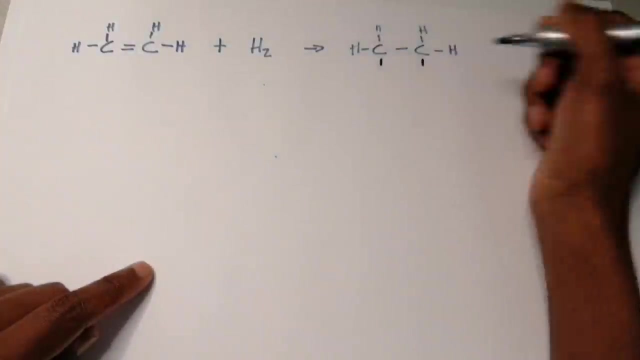 okay. and so what happens when it breaks? okay, so you had, we had that. and then remember the double bond. the second bond broke, and then now we've got two arms that are available, isn't it? one i'm there and one i'm there. and what happens? so those hydrogens. 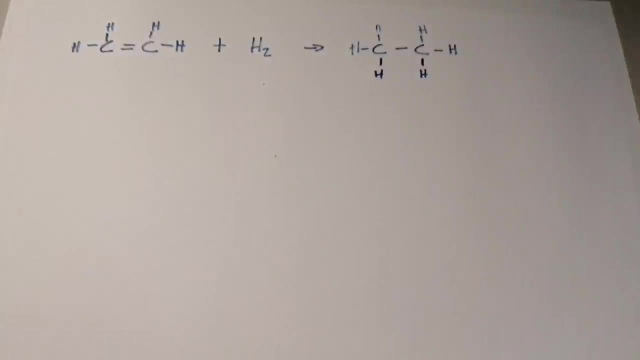 simply just go and attach themselves right there. okay, right, and then. so we moved this reaction from being an unsaturated hydrocarbon to being saturated. and what type of reaction is it? now, it's still an addition reaction, right? what type of addition reaction is it? it's going to be? 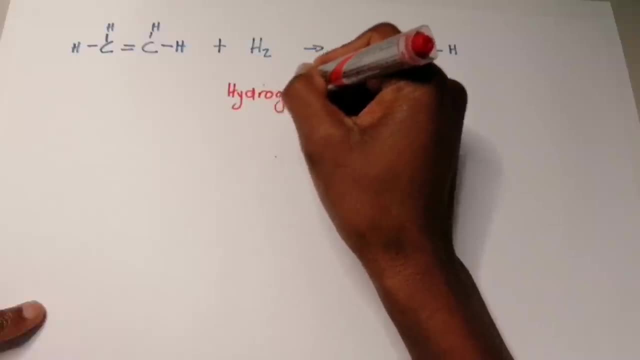 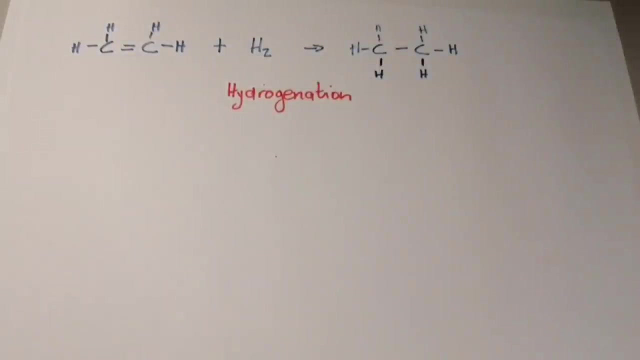 hydrogenation. we are adding hydrogen, so we call this hydrogenation. okay, right now. um just something that i want to uh, show you quickly, all right, um a principle or a rule that we call macaw nikoff's rule. okay, right, so so let's say, for argument's sake, we're going to take just 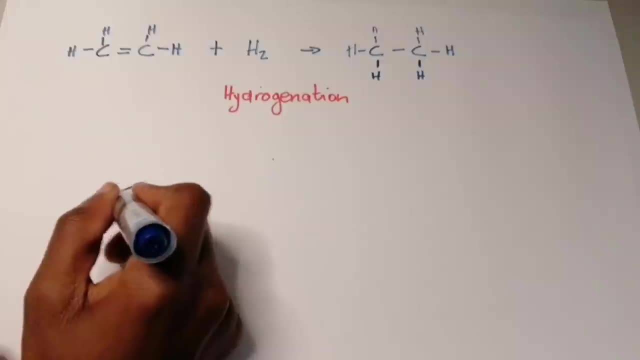 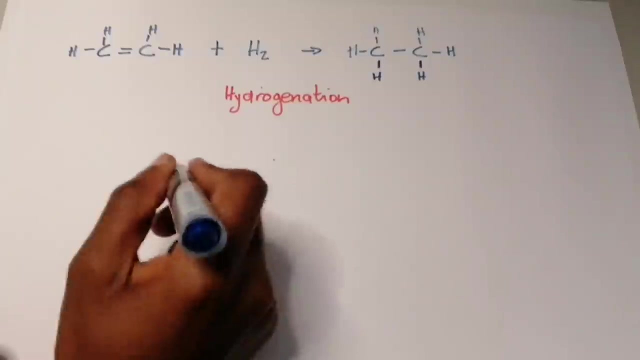 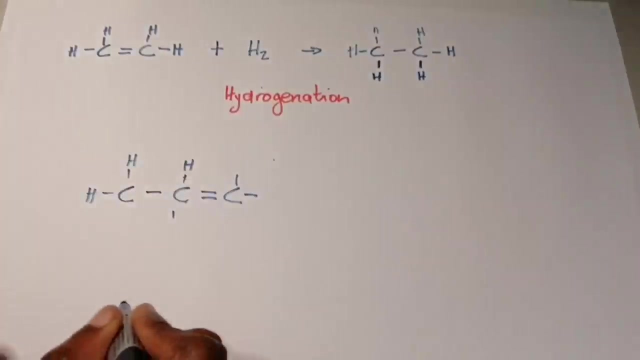 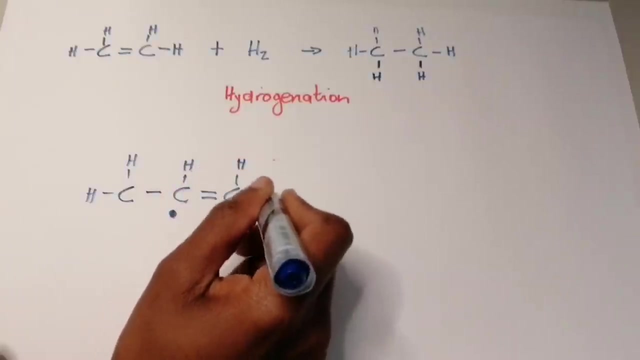 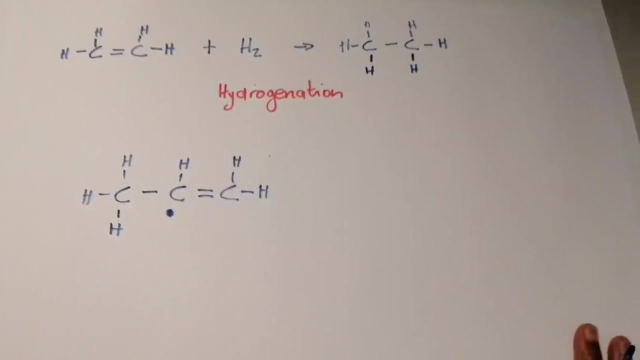 something a little bit different. okay, so let's take an alkene, unsaturated hydrocarbon. okay, yeah, let me take something like that. okay, right, and we're reacting it. um, all right, i've added an extra there, sorry, okay, so we are taking. okay, there we go, all right, so that's the proper one. so now we are taking. 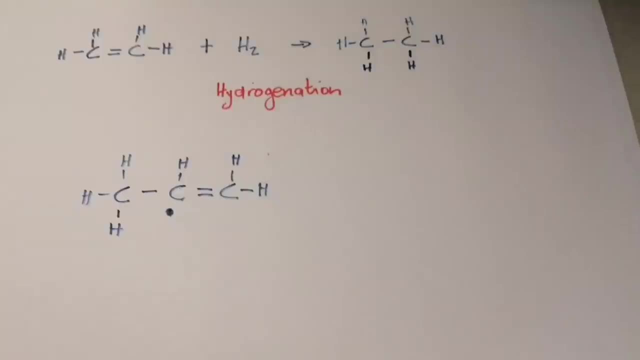 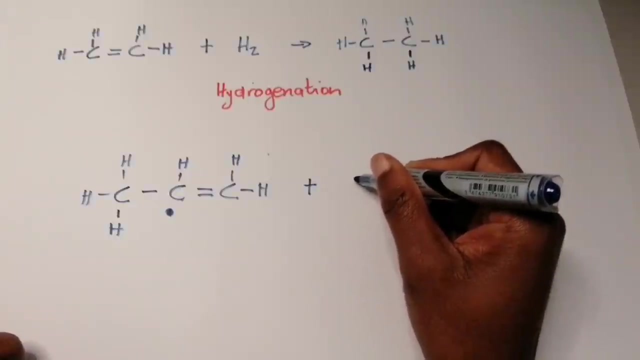 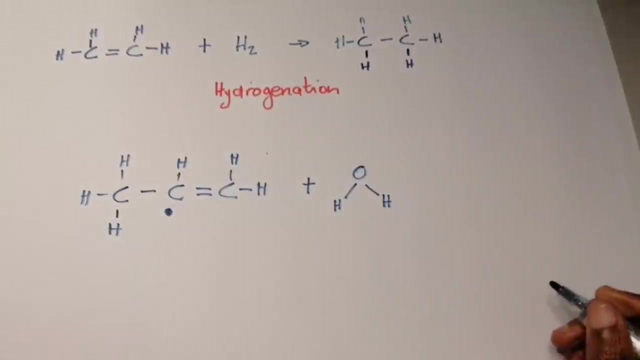 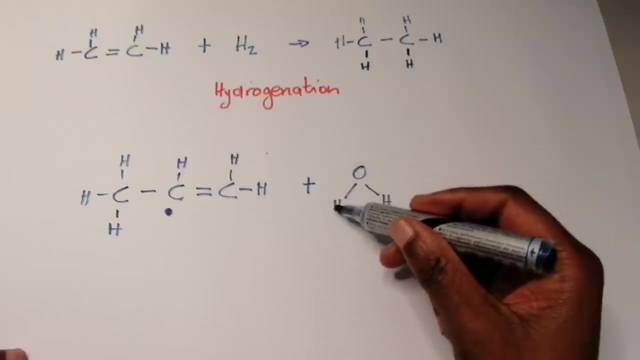 that um, alkene- and let's now react it with water- h2o. okay. so when you react it with h2o- in fact let me write it in structural form- okay, so we are reacting it with both sides. really see that it's actually'm actually reacting with H2O. now what happens is that H2O will. 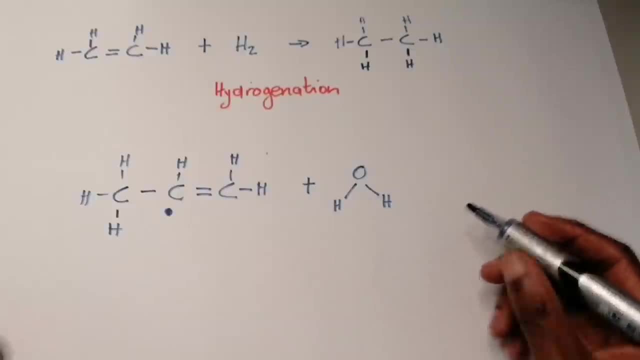 break down into 2, so H and uh o, h minus and H plus, right, and so what happens in this case? please, i want you to listen carefully. okay, so now we know we're going to have a substitution reaction, so we've got two possibilities, okay, okay. 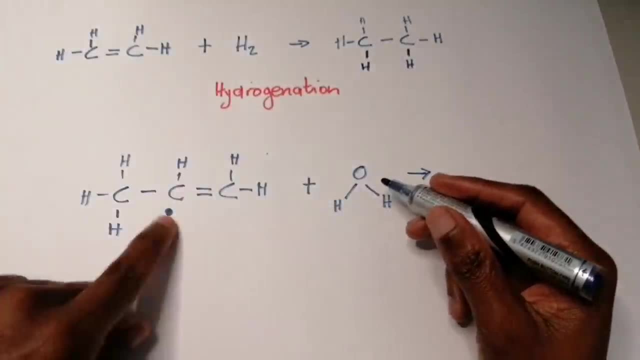 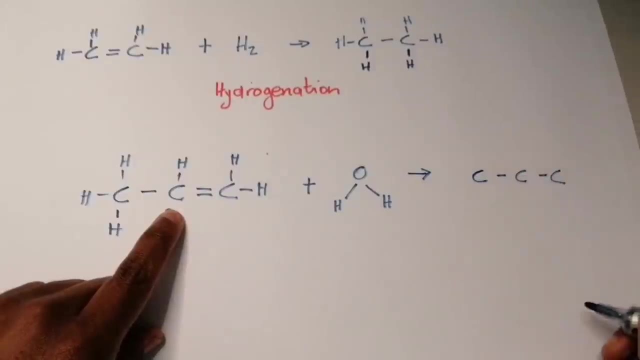 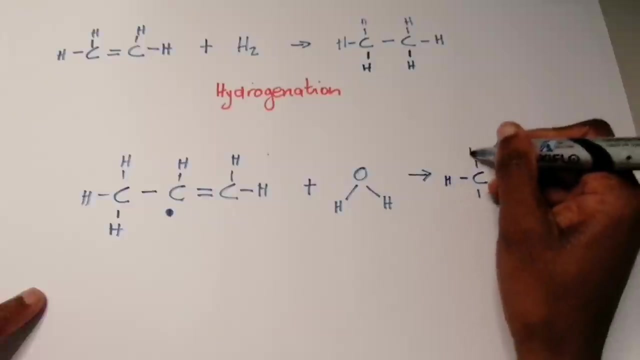 so the question is: where does the oh go? do we take the oh and put it, remember, when you go that other side? okay, so there it is. it's it moves from being unsaturated, okay, and it is now saturated. so we, we have that, so i'm just putting everything else there. 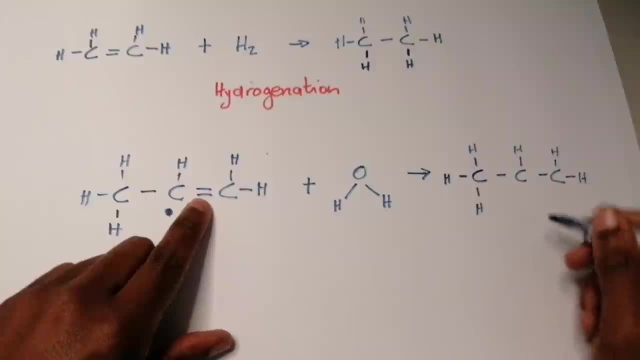 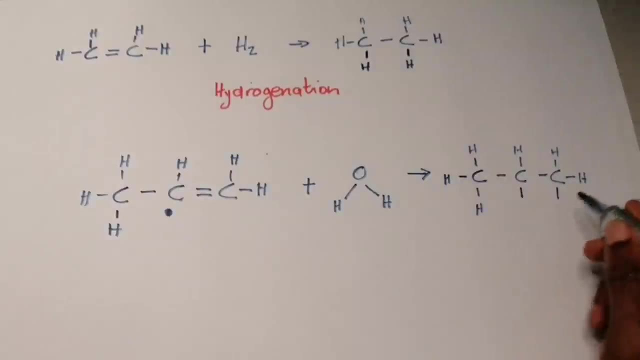 okay, that double bond breaks now. you've got those two spaces available right now. the question is: am i going to put oh here or an h there, so oh and h- or is it going to be the other way around- h and oh right now? then we talk about what we call the major product. so we've got two things. 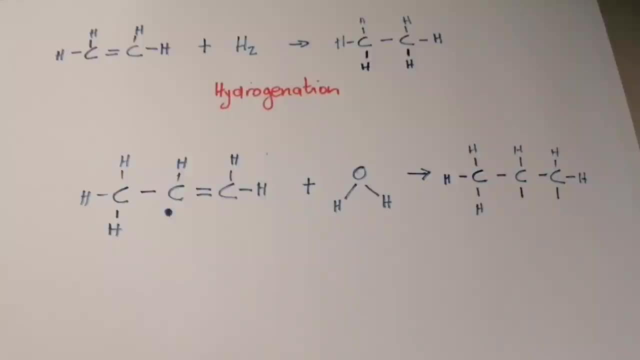 we've got a major product and the minor product. what a major product simply is is, in this type of reaction, most of the molecules that react with water would form a certain type of compound. that's what we call the, the, the, the major product. okay, so now this is where we're going to apply what we call mcconnickoff's rule. 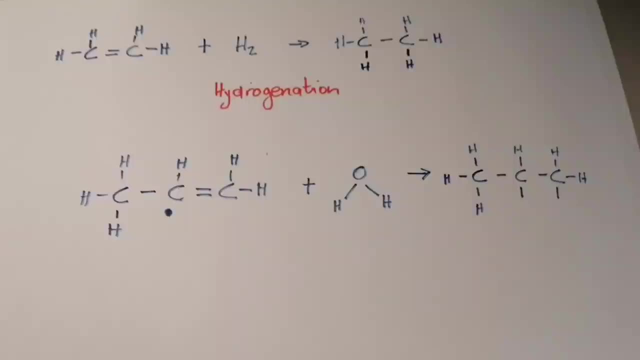 okay, and one more conical's rule simply says is that in an unsaturated hydrocarbon, if there's a reaction between hydrogen and something else- so it could be hydrogen and a halogen right- the hydrogen will tend to go to the carbon that has the most number of hydrogens. please, i want you to note what i've. 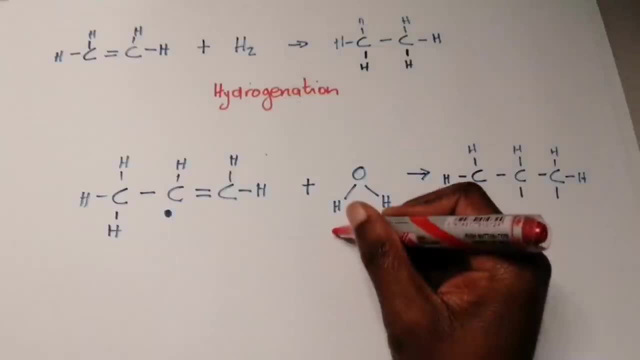 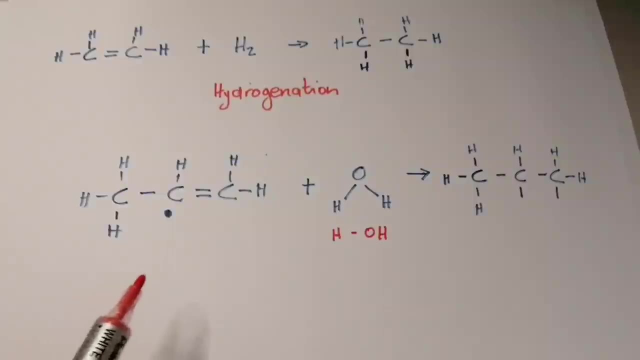 just said. so now we are going to have a reaction between hydrogen and something else, so it could be a mon statistical principle. we have one of theseeron SO masters. so theisiejs will have what h and oh so l his ruciones. the hydrogen will tend to go to the carbon that has the most number of hydrogens. now, please, i want You to. We'll have a combination of high and low, and low, but also f and low. no two carbons that are attached to it. can you seeause? there are a lot of thesemanpedial midday see right, and this is the case that happens when you go over here and you haveias begin to go because you're thegom of the ones that Gam patients can go to. thebe RPM. since CS has become high, like we have Your hydrogen from 10 volume beat, have of it above that. 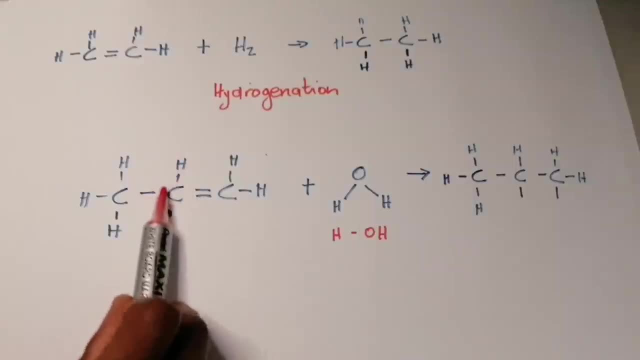 And then, if I look at this, how many carbons does it have? It has only one. So Makonikov's rule says hydrogen will want to go. The major product will be formed when hydrogen goes to the carbon that has the most number. 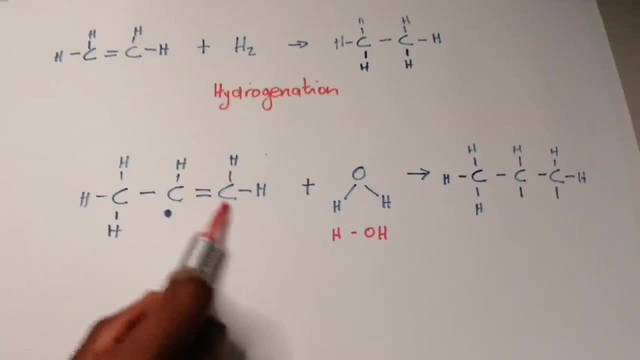 So this one is two, This one is one. So definitely hydrogen will tend to want to go to this one. So now, what we have as a product? okay, You will have a major product. This is what we'll call a major product. 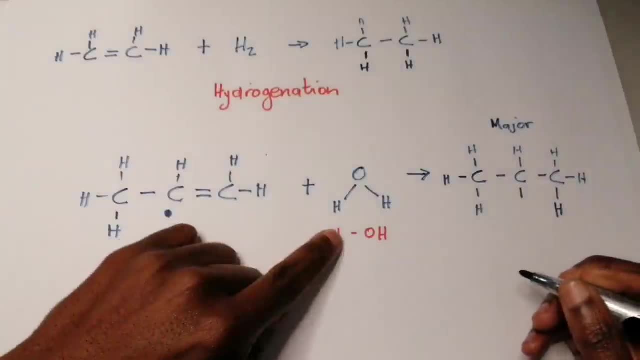 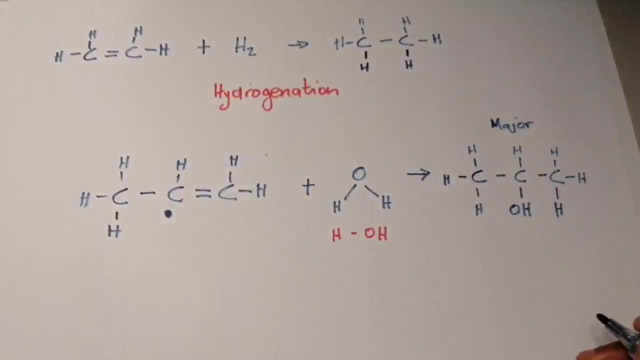 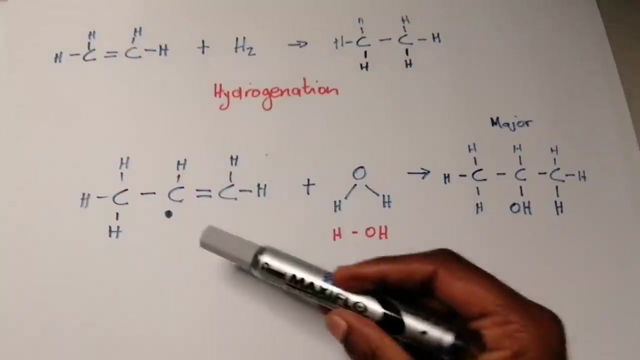 It means H will go there- okay, Go to that first carbon there- And then it means that OH will go to that second carbon there. By the way, this is the one way of forming an alcohol. Can you see that Right? 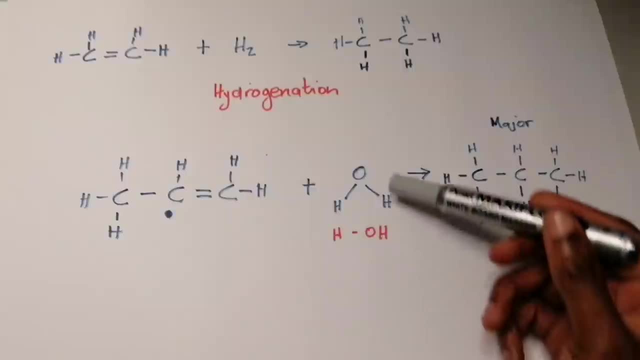 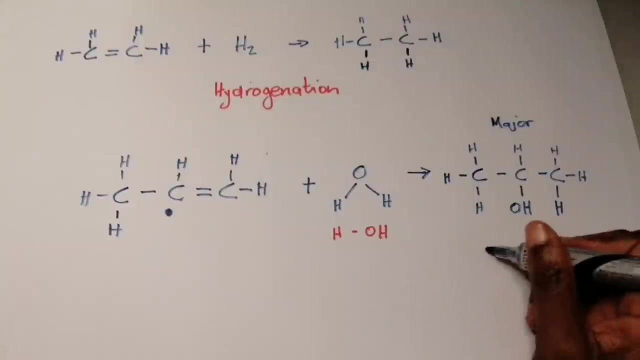 So what we've done is we've taken an alkene, We've reacted it with water- Water, okay, H2O- And now it has formed an alcohol Albeit. it's a secondary alcohol for the major product, So it means that your minor product therefore okay. 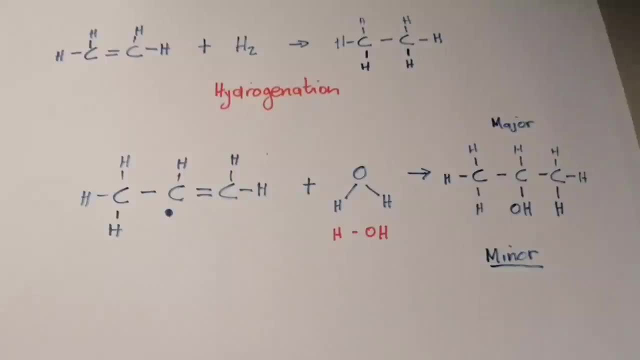 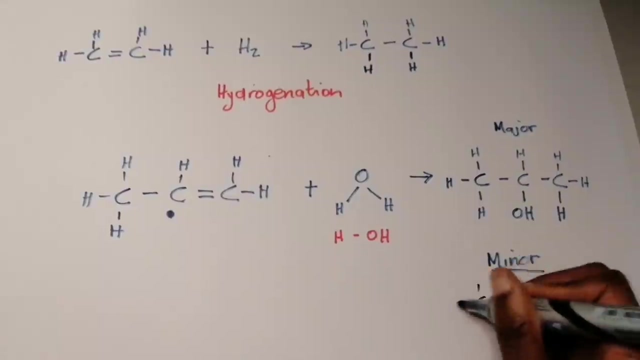 So if the examiner does not specify, you must assume that the product will be the major product, right? So it means that your minor product will be So in this reaction. it means that your minor product will be the other way around. So H will go there and then OH will actually go to the first carbon. okay. 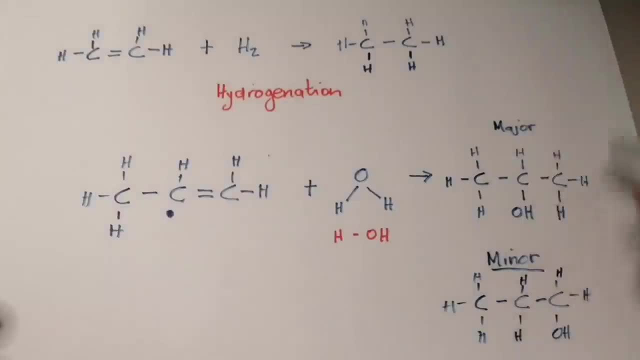 So most of the molecules actually will form that product there. That's why we call that the major product. okay, Right, so that is what we call Makonikov's rule, right, Okay, Okay, Just note that quickly, right. 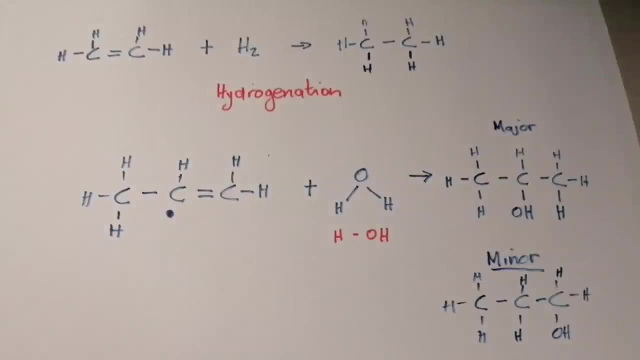 So we said the hydrogen tends to go to the carbon that has the most number of hydrogens. That is how our major product is formed. And, by the way, what type of a reaction is this? Once again, can you see? it's an addition reaction, right? 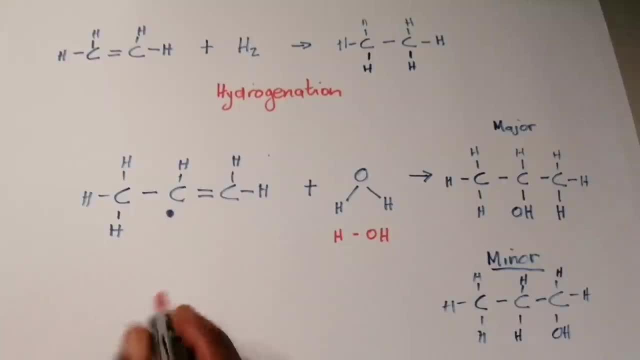 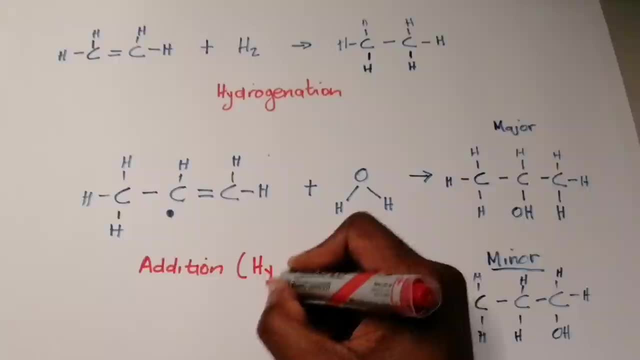 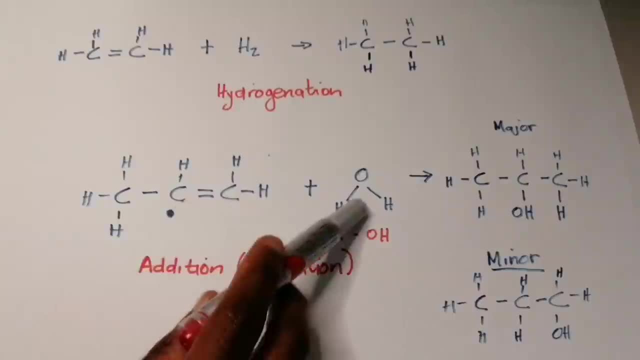 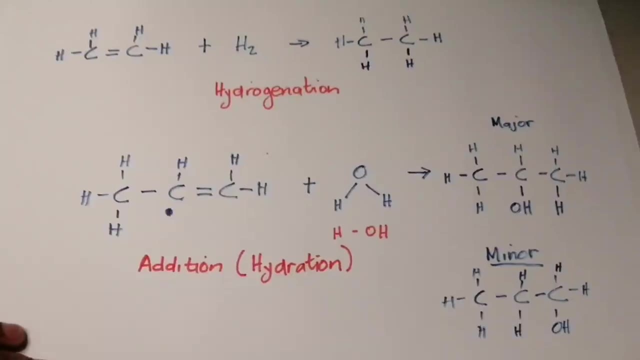 So, in this case, what did we do? We reacted this with water, So this is what we call a hydration reaction. okay, Right, so where an alcohol is formed, All right. Okay, let's go on to the next one. 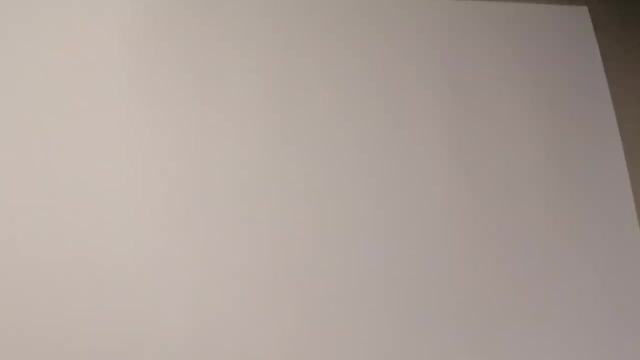 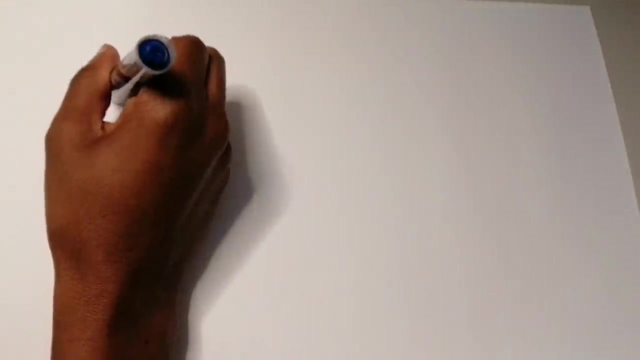 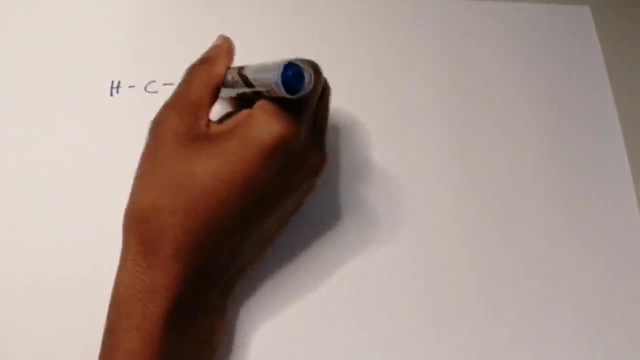 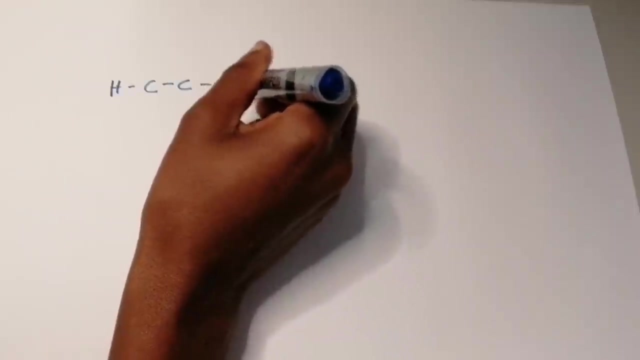 Just, I want to show you just another application of mcconnick of the rule. okay, so say, for argument's sake, we've got right, let's let's take another compound. okay, all right, let's take something a little bit bigger so that you don't okay, so let's take, suppose. 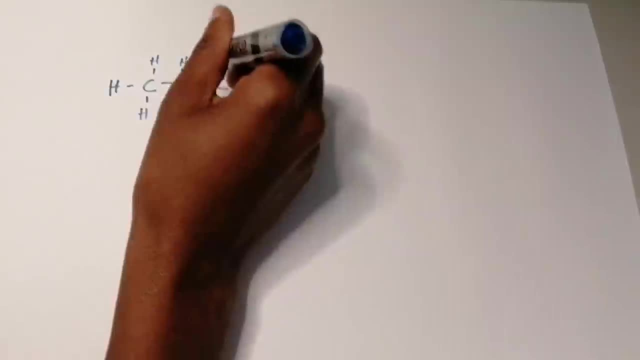 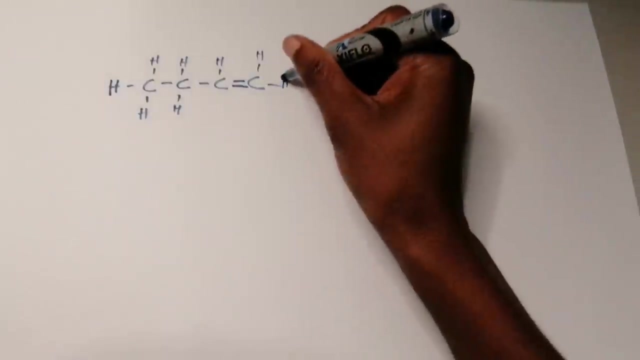 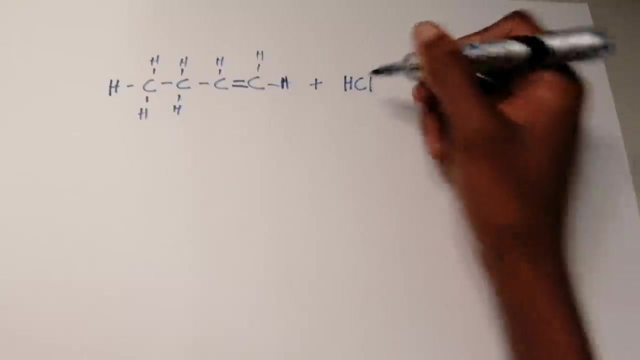 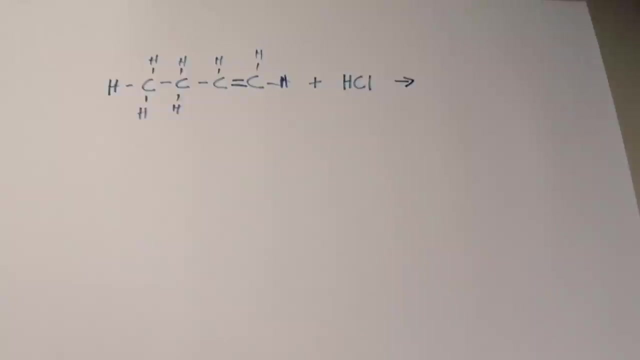 we've got butane butane, right, okay. so with butane butane, nah, butane one ene, rather okay. so we're going to react that with hydrogen chloride. okay, can you see. so it's not a halogen. okay, right, so in this case it's. 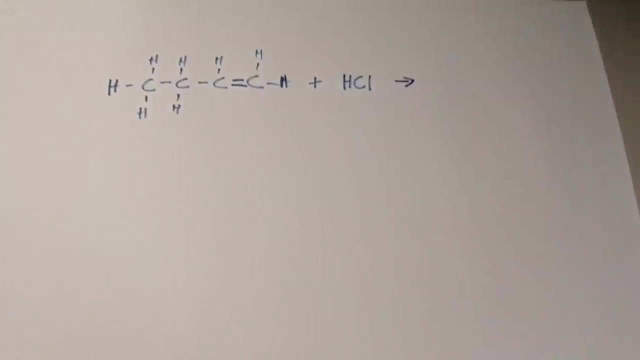 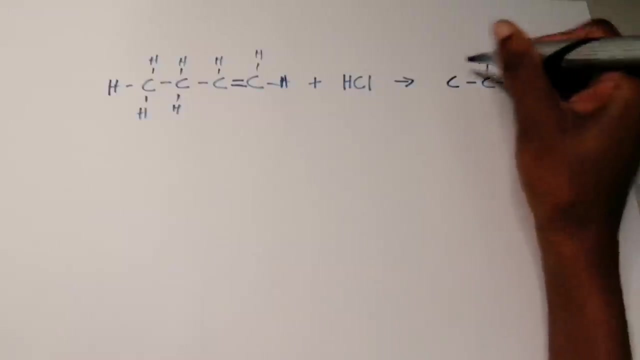 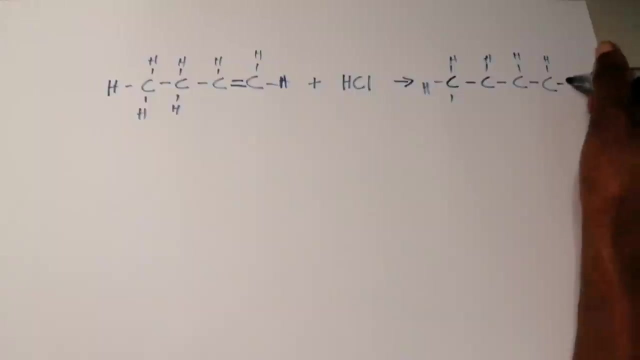 hydrogen chloride. So what happens? What is going to be the major product in this case? So once again, we're going to apply Makonikov's rule for the major product. So what happens? So we're just going to simply say OK, for this one, we have HCl. 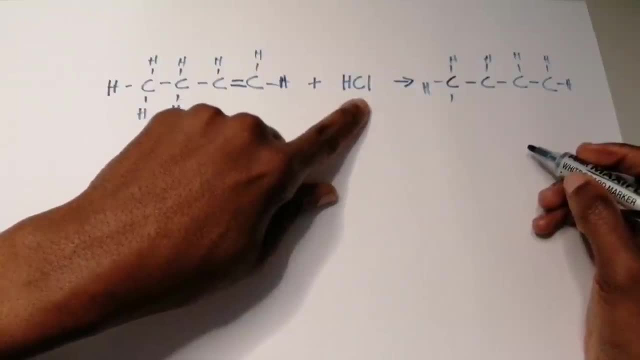 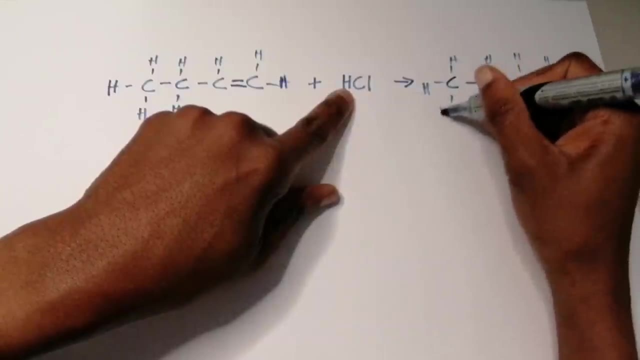 So it's hydrogen and the chloride ion, Right. But what does Makonikov's rule say, Right? So now there's hydrogen hydrogen there, So double bond breaks, Right. And then we've got two spaces available, Right. 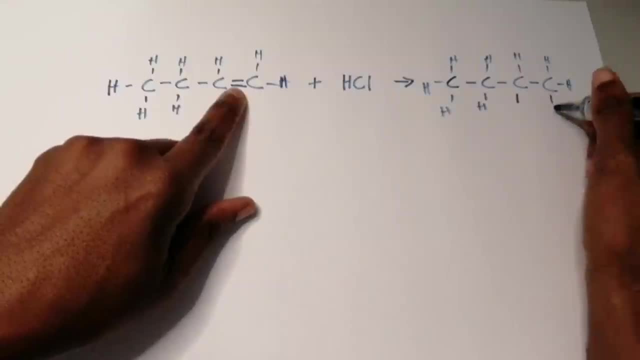 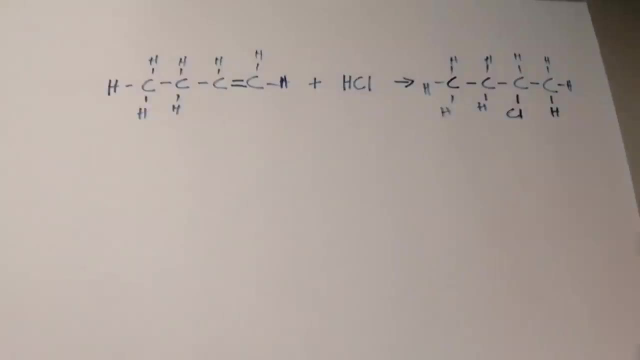 So the hydrogen goes to the carbon that has the most number. So hydrogen will go there and this will be the chloride will go there. So in this case this will be 2-chlorobutane Right, Whereas this was but-2-ene. 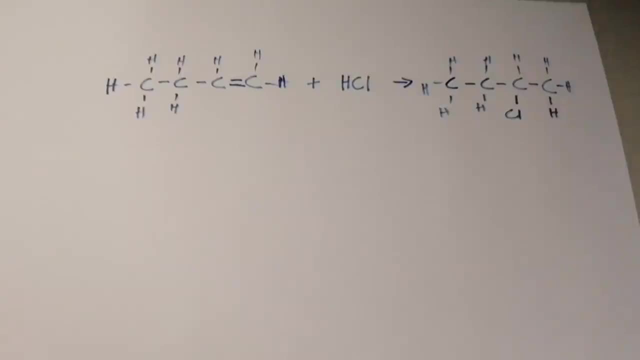 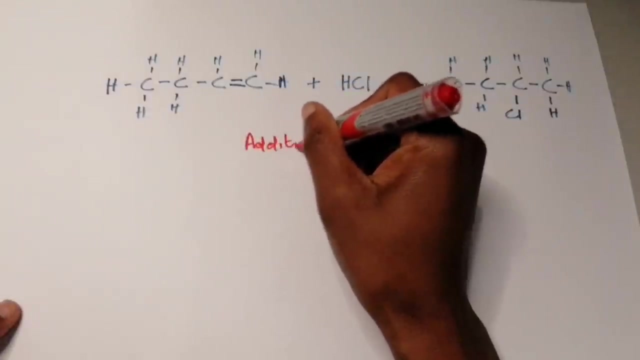 I hope That makes perfect sense, ladies and gents. By the way, what type of reaction is it? I'm sure you've got it by now. This is once again an addition reaction. OK, But what type of addition reaction is it? 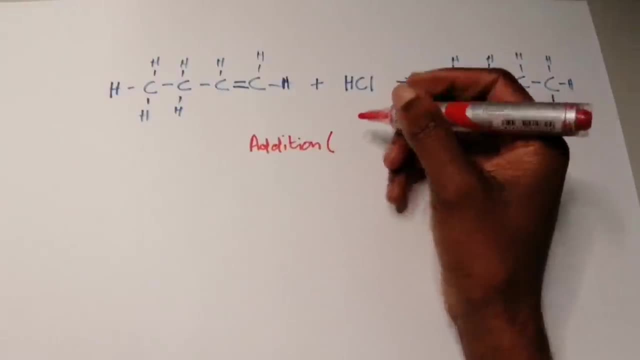 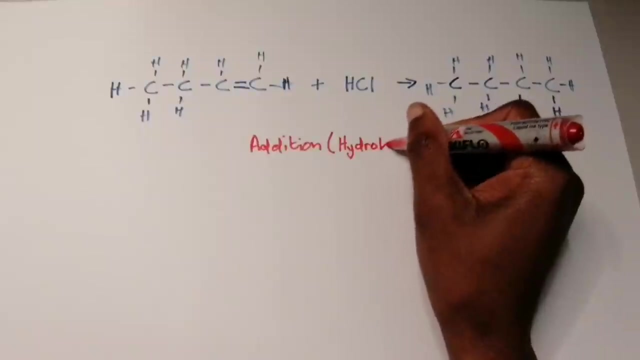 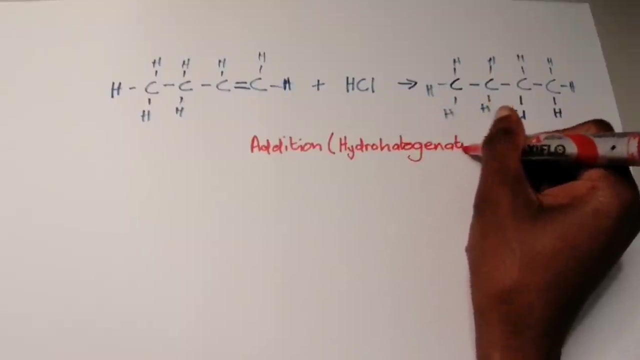 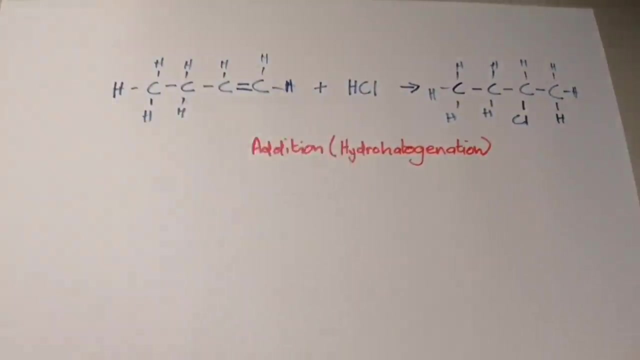 Right. So once again it is what we call in this case Hydro Halogenation, Halogenation, OK, Hydrohalogenation. So two things reacted there. It was the hydrogen as well as the halogen, OK. 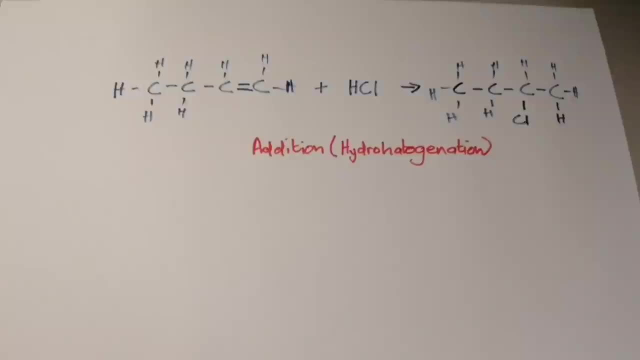 So those are the types of reactions that takes place. OK, Right, Very quickly, let's go through another one again. OK, So we've got another type of reaction that takes place. OK, So in this case, this is what we call A. So we've gone through substitution, we've gone. 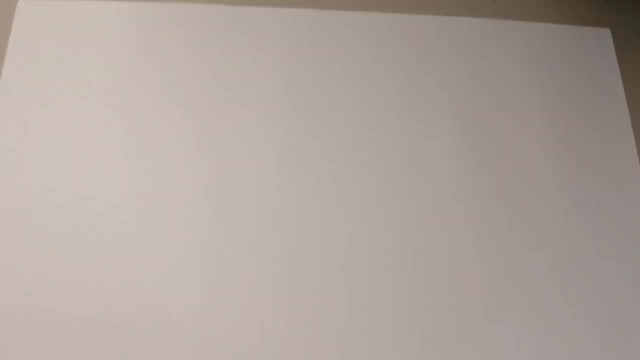 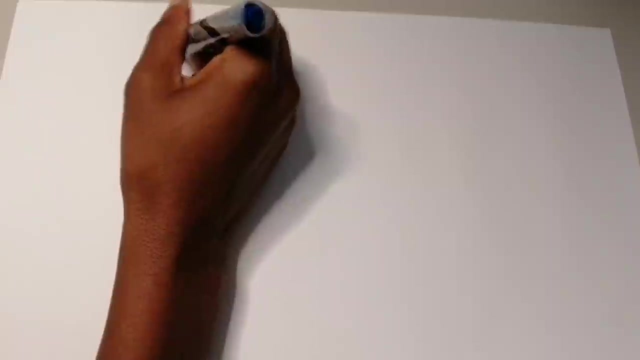 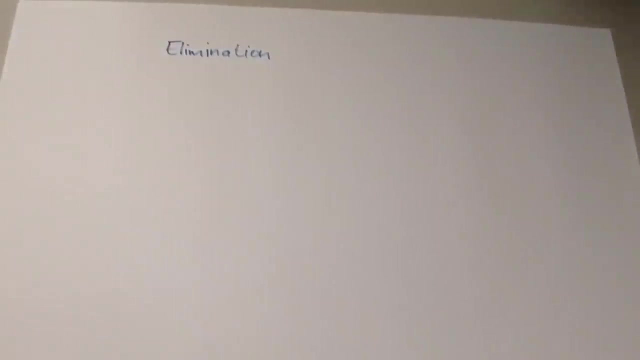 through combustion. we've gone through addition reactions- right, So we take what you call an elimination reaction. OK, So, we do have what you call elimination reaction, OK, Right. So, as the word suggests, right, you are eliminating something. 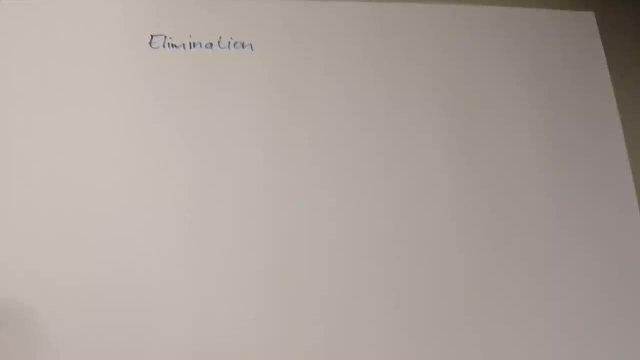 OK, So what happens in an elimination reaction? OK, So you are taking something that wasn't there. OK, Let's just focus this a little bit. OK, So you are taking something that wasn't there and you are now sorry, rather removing something. 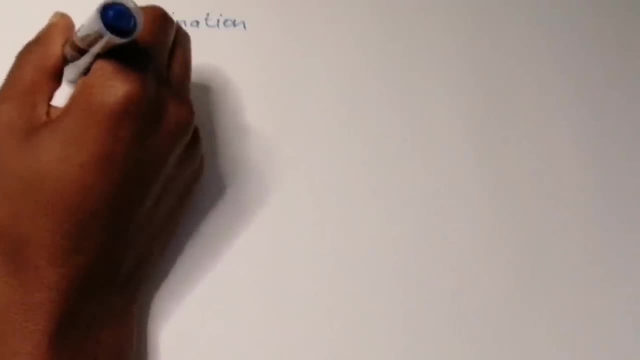 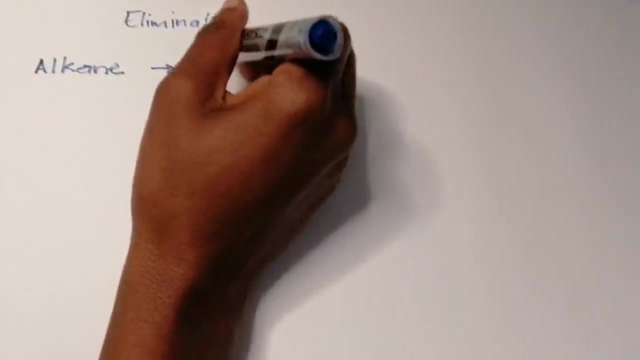 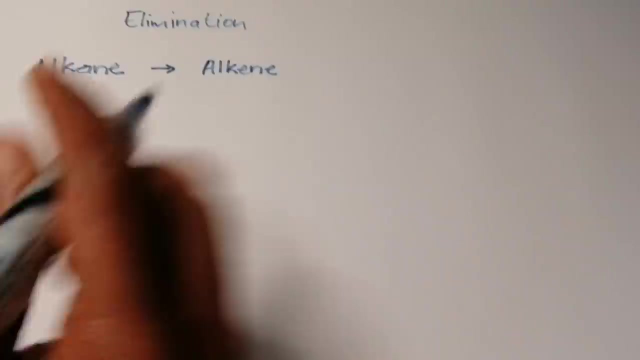 that was there. So you've got two types. that can really happen or that can really take place. So you can have an alkane. OK, That can form an alkene- OK. So you've eliminated something. or sometimes it can be more than one, so it could be alkenes. 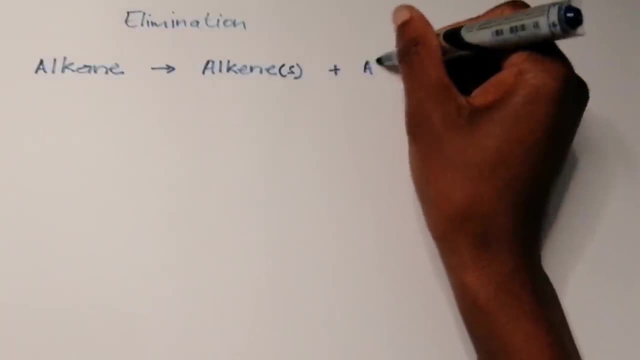 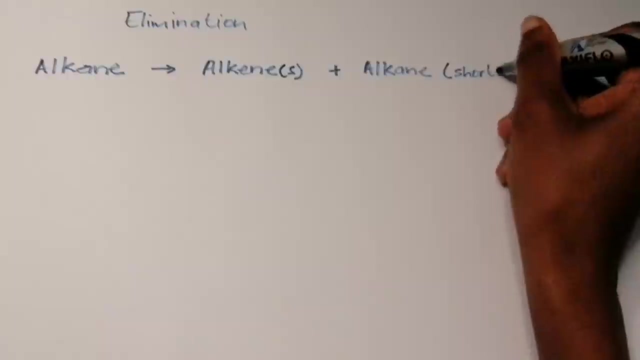 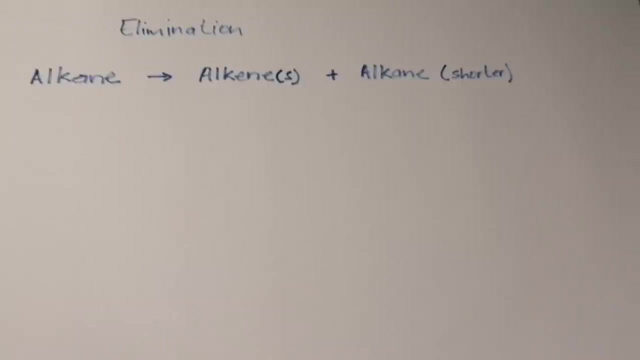 OK Plus another alkane. I'll show you what I mean by that. OK Plus another alkane. Right, Usually something with a shorter chain. OK, Right. So that's what happens in your, in your elimination reaction, or even, at times, you may have a situation where you take an. 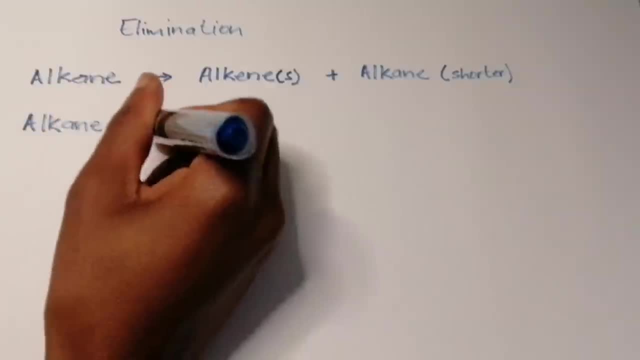 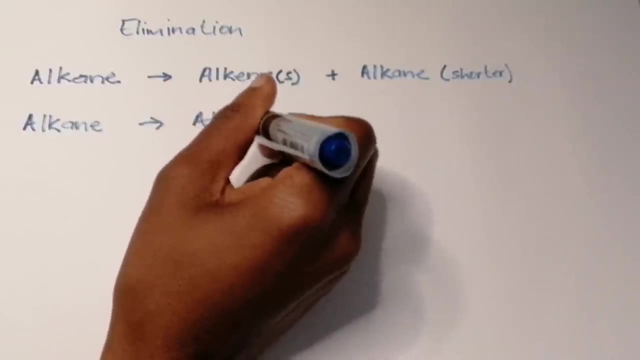 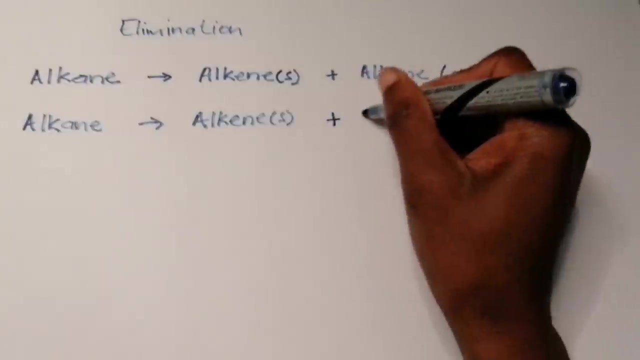 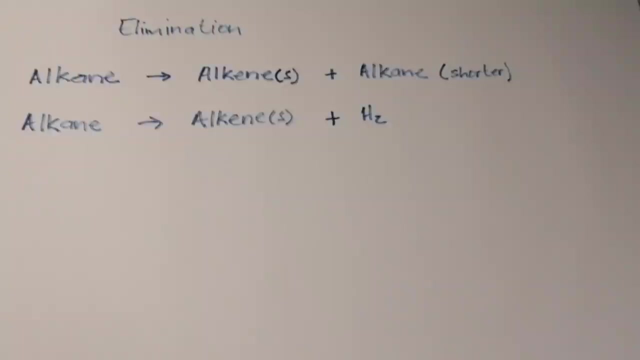 alkane, all right, and it forms an alkene, or it forms alkenes, okay, and hydrogen, all right. so that would be a typical situation of an elimination reaction and, by the way, I just want you to note there, okay, you wouldn't necessarily know what products are formed. 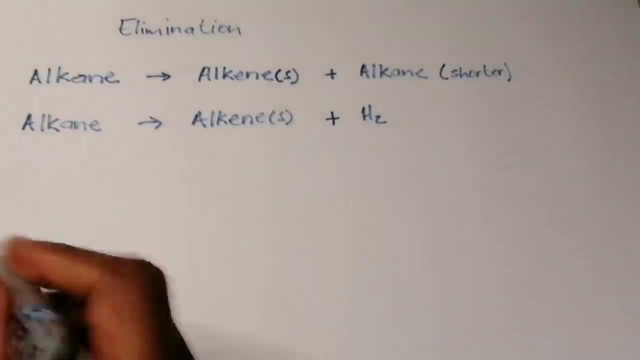 okay, all you need to be able to know is apply it in a situation as I'm going to show you just now. so suppose we take something that simple. okay, so let's take a effect. you know what? let's do this. 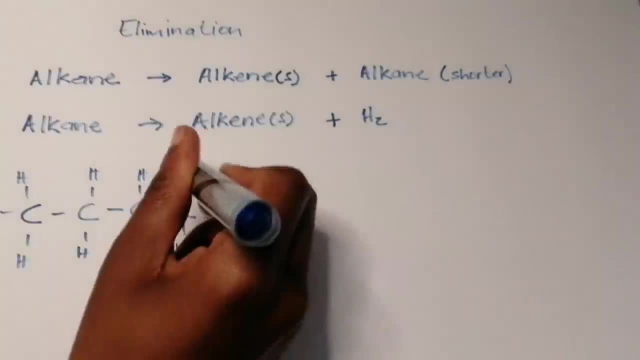 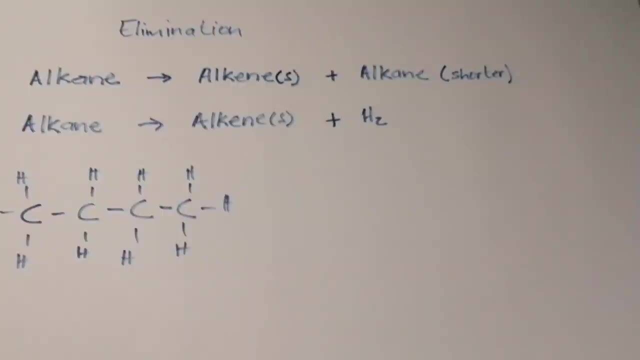 so let's take an alkane and we say we are going to take it through what we call an elimination reaction. right, so undergoes an elimination reaction. and in this case, what happens in that reaction? okay, we said, we can have. 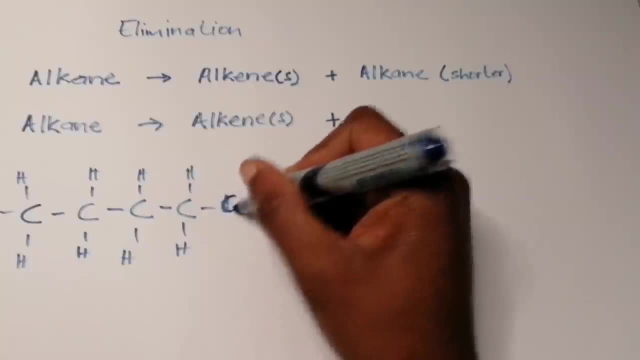 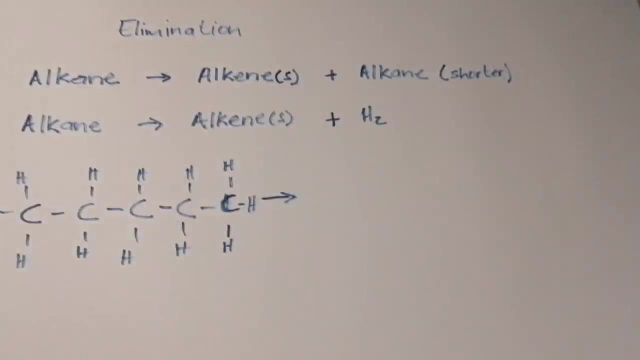 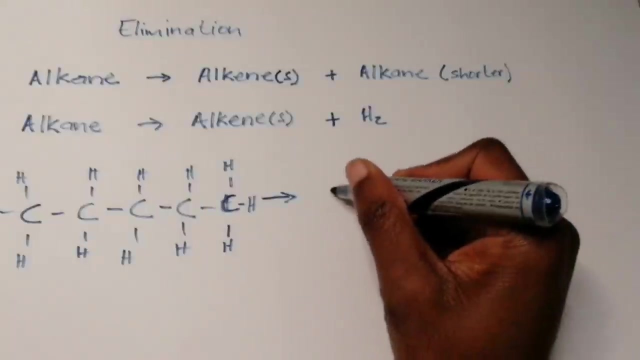 in fact, you know what? let me just make that a bit longer. let me just add another hydrogen so that it could make for a more interesting product. okay, so let's take, this is pentane. okay, so now one of the products that you can form is: 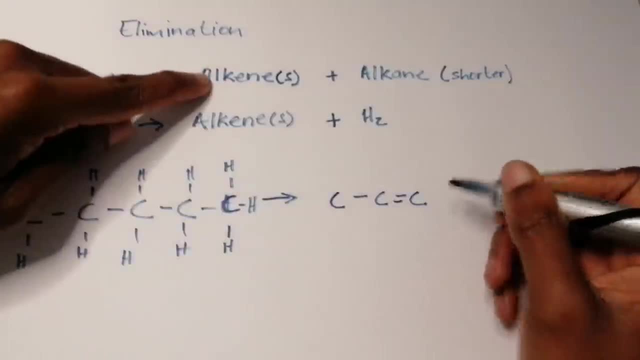 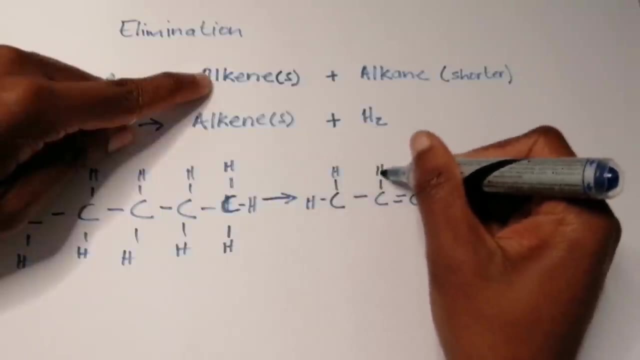 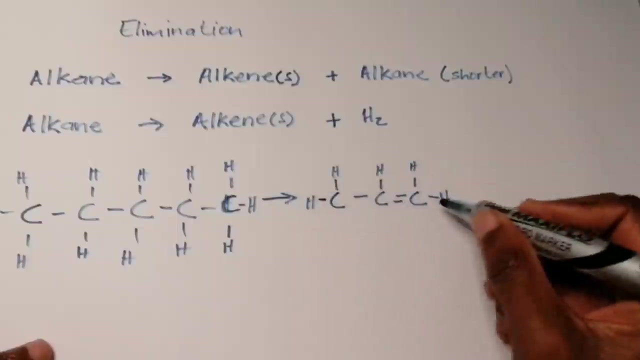 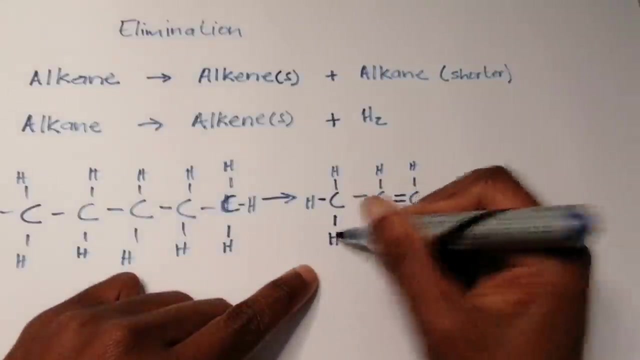 we said an alkene, right, please I want you to note, so we can form an alkene right through an elimination reaction. okay, and what happens now? please I want you to note. how would I know? and usually when they ask you this, they'll say: it will form this and let's. 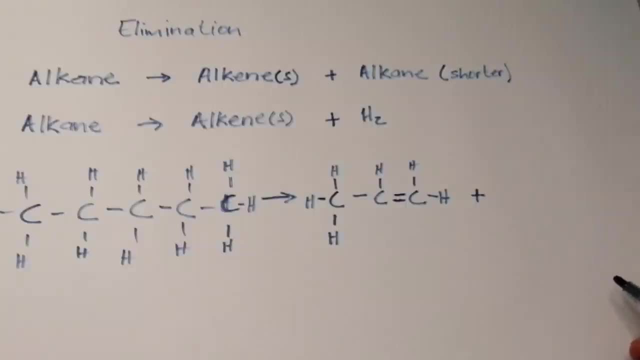 say product X, and then they say: give the structural formula of product X. okay, so now what is still missing there? you've got an alkene. we had an alkene with how many carbons? one, two, three, four, five, right, so now, on the right-hand side, how many carbons do you have? 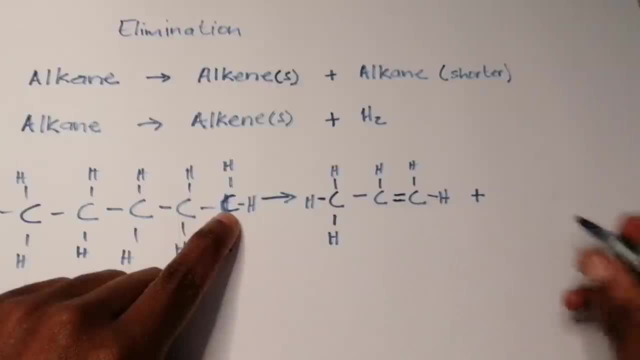 one, two, three, right. so how many are missing? two? so now I know I'm going to have another carbon there, right? and then hydrogens I would have had. so the number of hydrogens there. 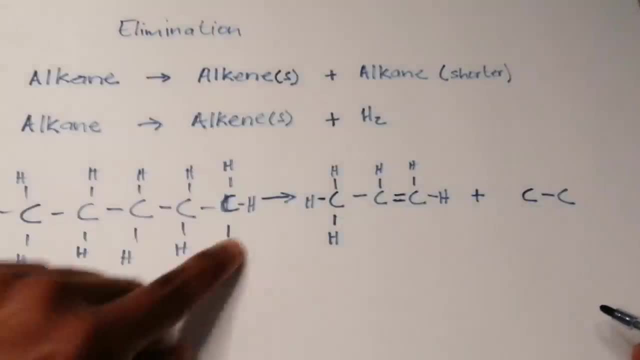 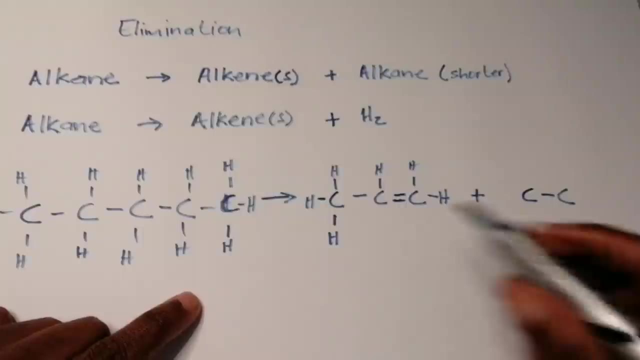 that's three, that's five, seven, nine. okay, that's 11,. sorry, that's 12, right, so now you've got 12 hydrogens. how many did you utilize there? that's one, two, three, four, five. 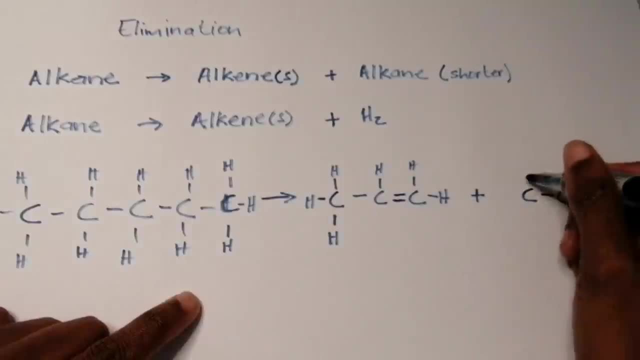 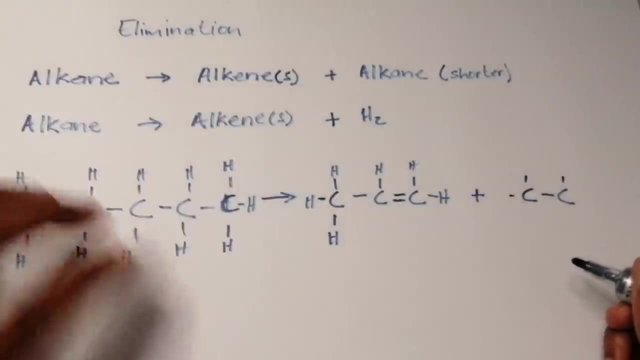 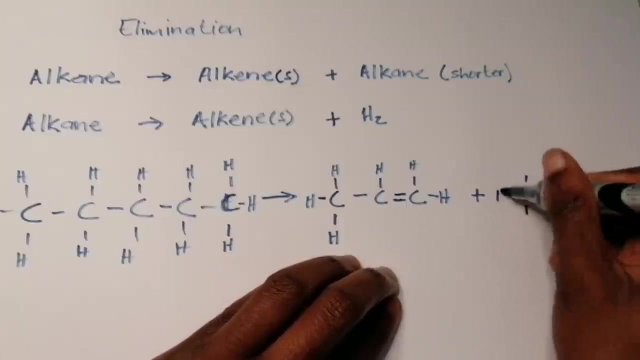 six. okay, so how many are still missing? okay, right, I'm clear that you're getting it. so you still have six. so you had 12 this side. you used six over there, so it means that you need six more. so in this case, I'm going to have something that looks: 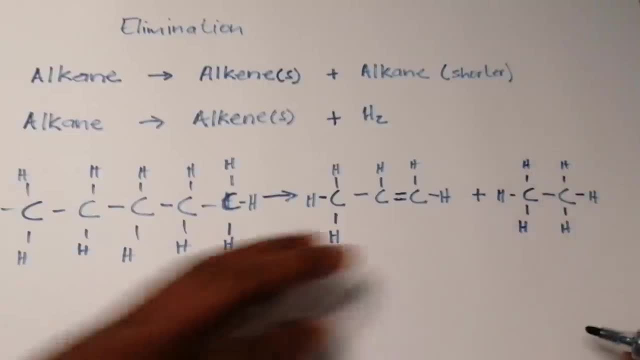 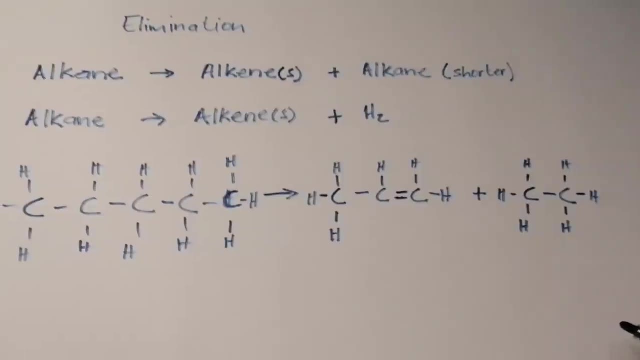 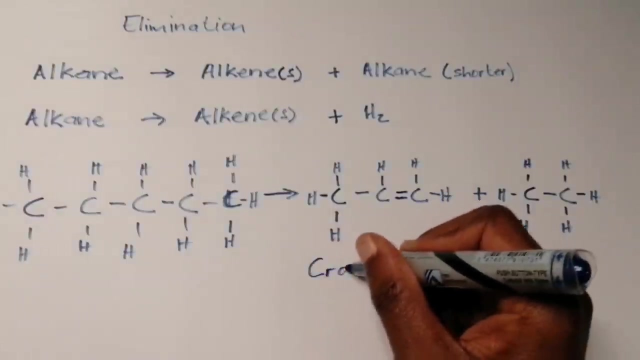 like that. okay, right, so that's the first type of elimination reaction that you're going to have. okay, by the way, sometimes they call this process. they call it cracking, right, cracking. so what's happening? in cracking, you're breaking down large compounds. 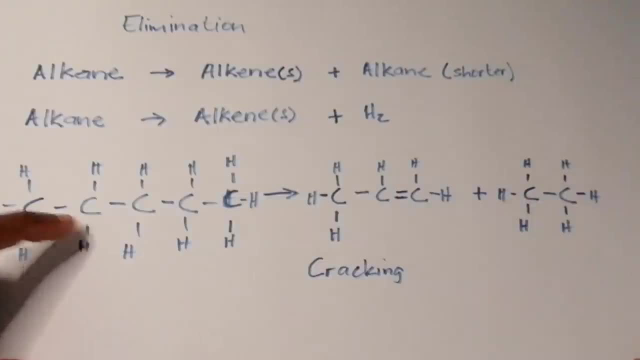 you are now breaking them into smaller ones. okay, by the way, when they get crude oil, it's a very large organic molecule, but they break it down into smaller ones. okay, in this case, that's where petrol is formed, that's where jet fuel is formed. 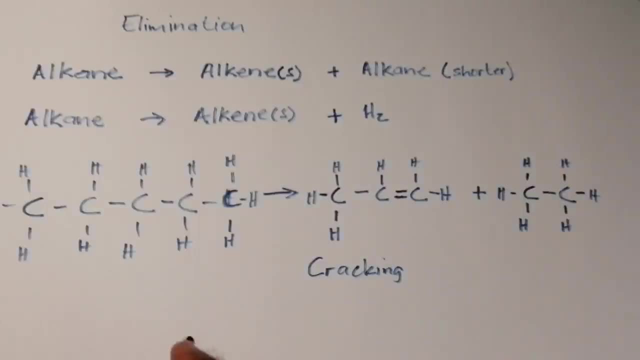 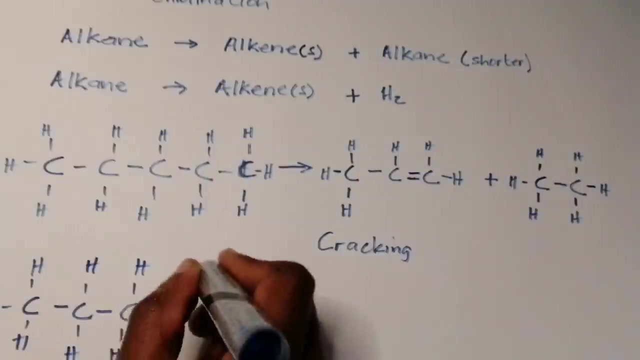 and all of that. right, they are smaller compounds, they are more usable, okay, so another type, okay, right. so there you go. you've got another reaction there, let's take, let's put that there. okay, right. so what else can we form? right now we apply a process there called Zaitsev's rule. 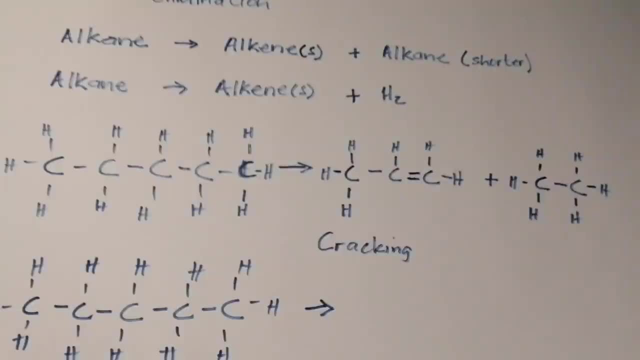 right and, by the way, okay, this is when you'll apply Zaitsev's rule, when you've got hydrogen and something else, but more likely is that hydrogen will tend to be moved or removed from the carbon that has the least number of hydrogens. okay, so you might form something like this: 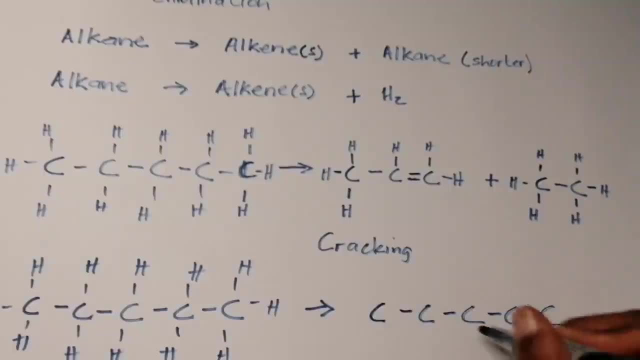 okay, you might form something that looks like that: with a double bond there, you could have placed a double bond there, you could have placed a double bond there. it's still the same thing, right, okay, okay, so it's this kind here that we're talking about. 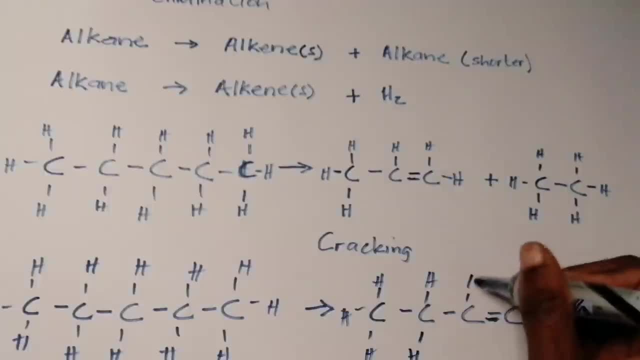 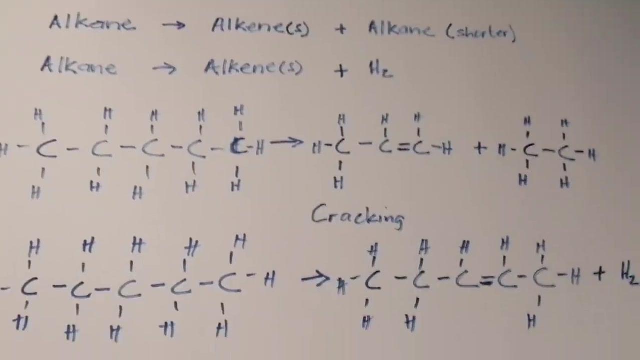 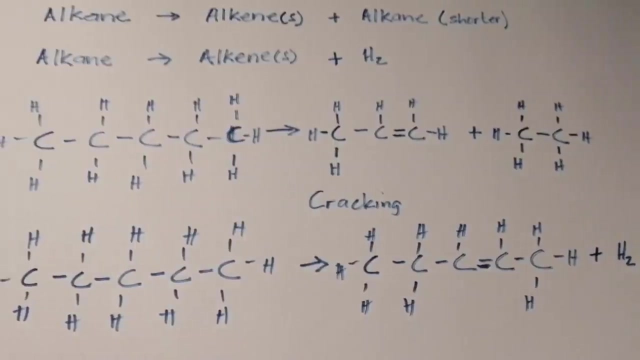 you form an alkene. okay, but your alkene also has- remember, we removed two hydrogens there and so this would be H2 there. okay, right. so in this case you moved the alkene and now you've got H2, okay, right now, just quickly. 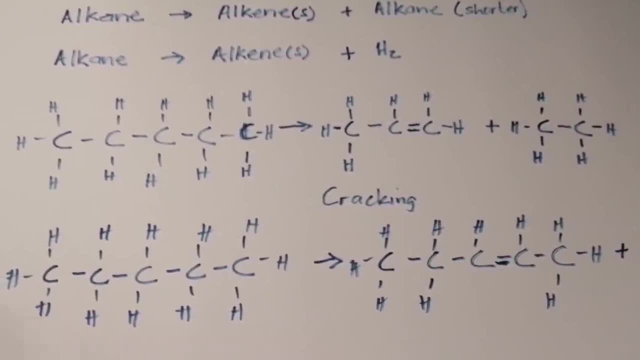 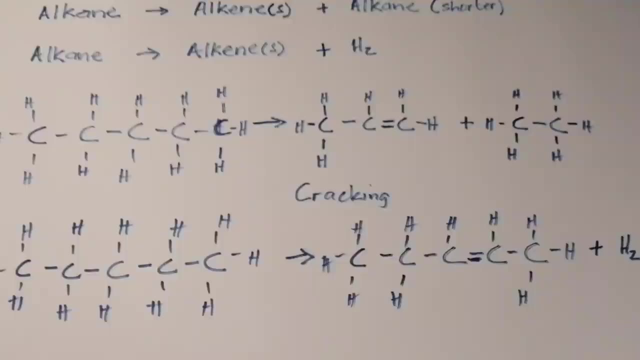 just to show you what type of reaction do we call this? all right, so we call this. this is an elimination reaction. once again, all right, but what did I remove? I removed hydrogen, all right, so this would be dehydrogenation. 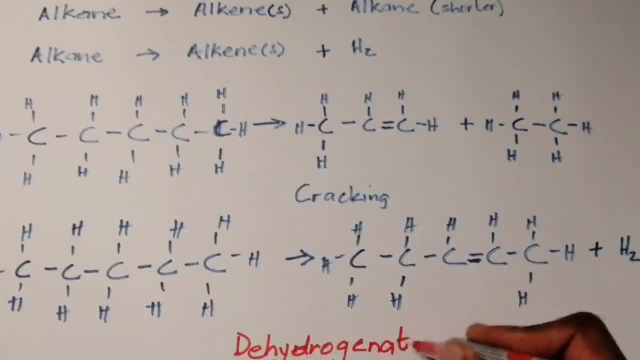 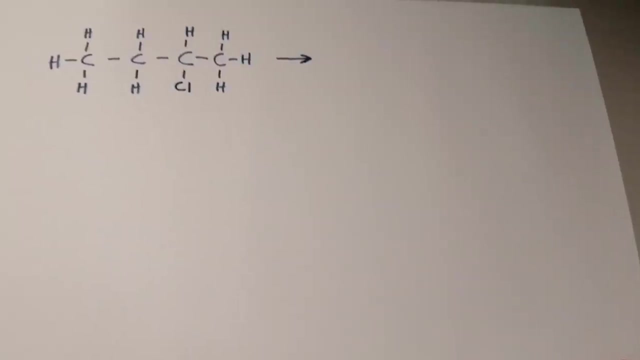 okay. so when I remove hydrogen- yes, it is an elimination reaction. this is dehydrogenation. okay, right, I hope that we're still together, right, okay? okay, just to show you again how to apply that Zetser's rule. okay, so we've got a haloalkane here and we are trying to make 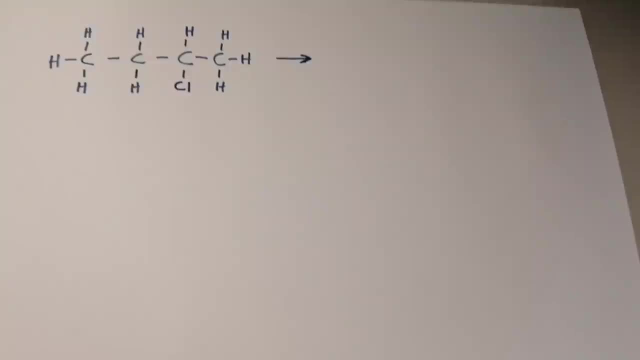 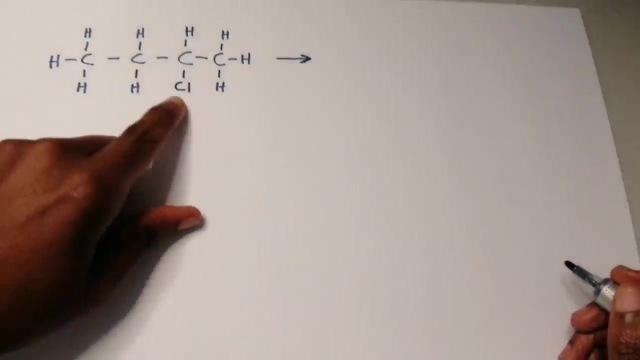 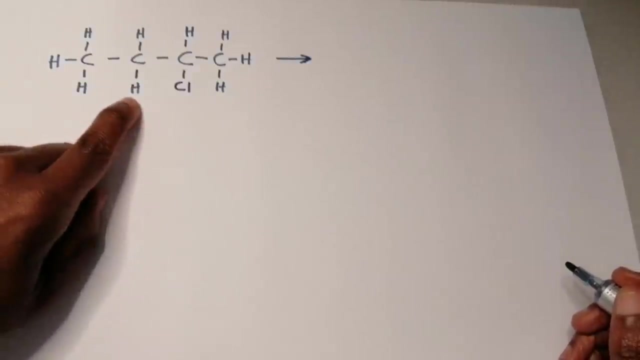 to have an elimination reaction, right. so what are you going to have? okay, so there are two possibilities. we definitely are going to eliminate that chlorine atom there, all right, but the question is, which hydrogen is it going to go with, this one here or this one there? and this is where we're going to apply Zetser's rule. 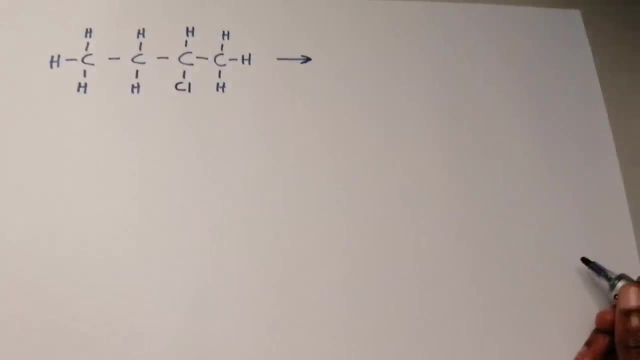 right and Zetser's rule simply says: in an elimination right the major product will actually have remove hydrogen from the carbon or will take hydrogen from the carbon that has the least or that has a lesser number of of of hydrogens. 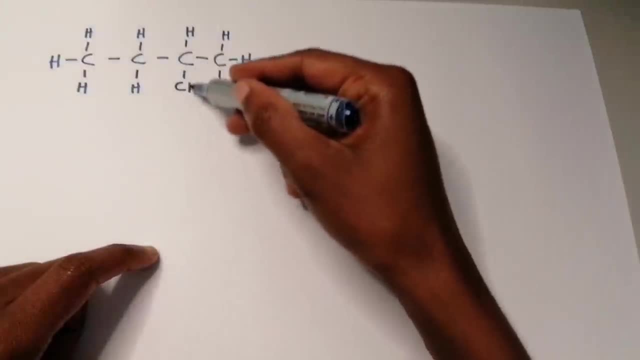 right. so if I look at this, I know definitely this one is going to go away, right? so let's check how many carbons, how many hydrogens. rather, does the Zetser's rule say: oh it's. 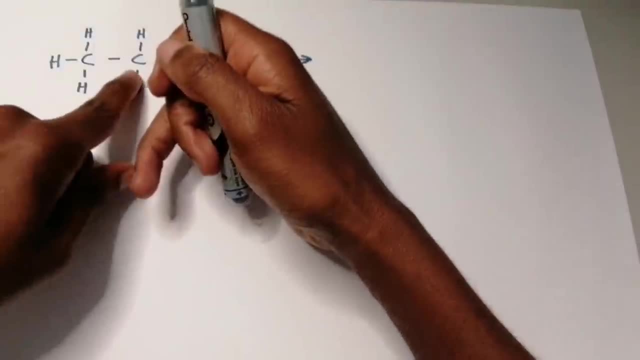 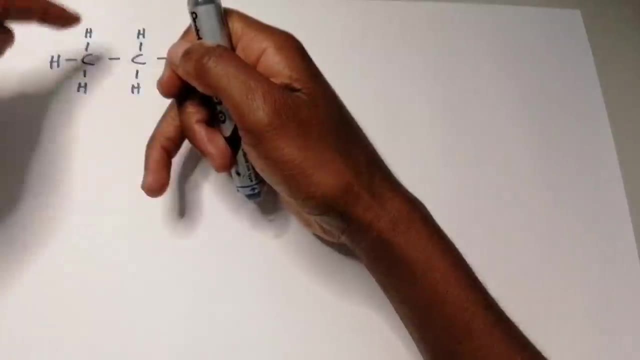 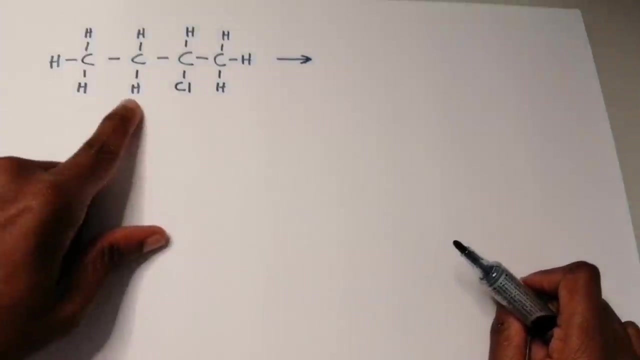 going to have. it has three right. how many hydrogens does this one have? it has two. so according to Zetser's rule, right, the one that has a lesser number of hydrogens will tend to forfeit its hydrogen. so definitely this one has a lesser number, right. so the major product will. 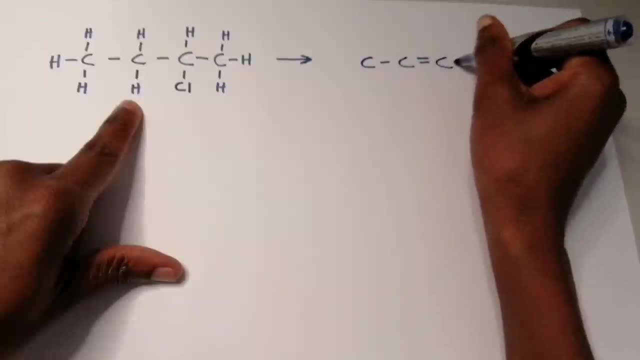 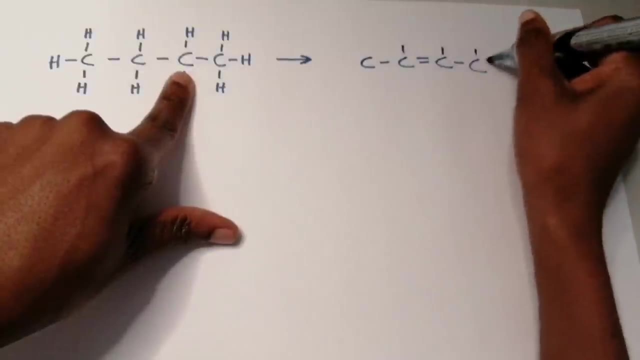 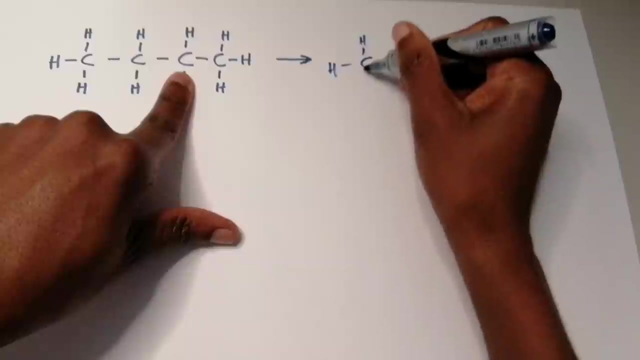 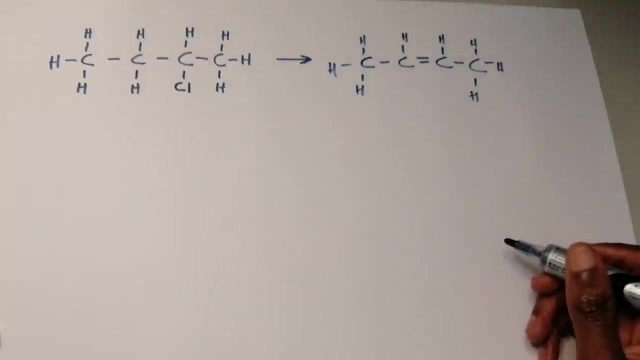 have hydrogen, so we'll remove this hydrogen here and we're going to have a lesser number of hydrogens here. we'll remove that chlorine there, okay, so remember, everything else stays exactly as it is. okay, right, so you'll have something that looks like this. okay, right, so you could have had that. 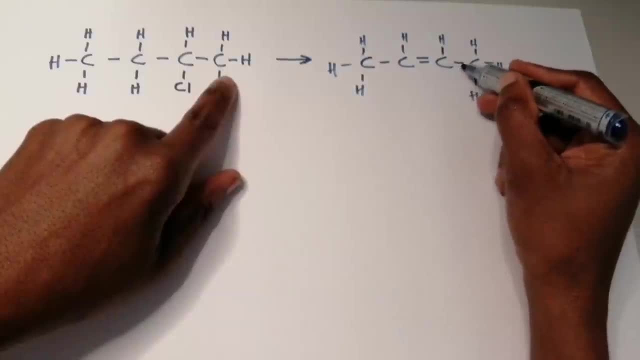 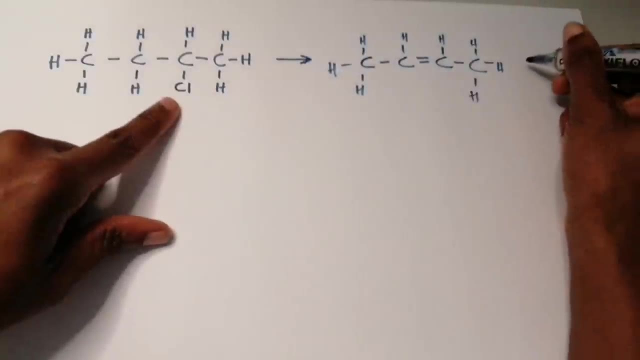 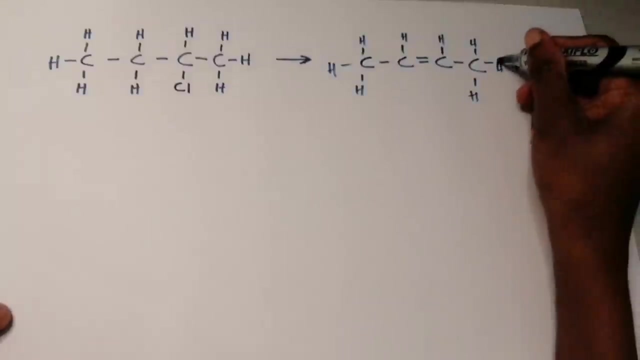 so obviously in the minor product you'll have a double bond there between the first and the second carbon, right. but now please just note we remove. we removed HCl, so in this case this would be plus HCl, just in case they want you to show. 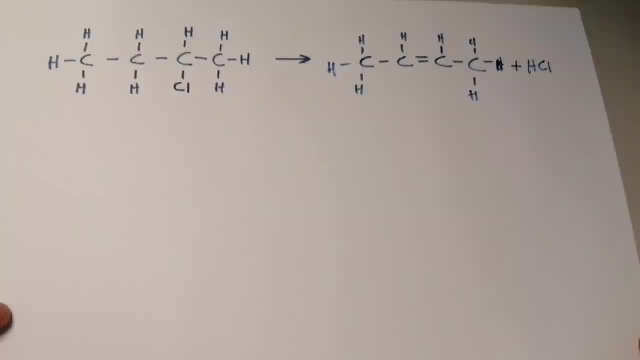 the reaction there. all right, so Zetser's rule says you take hydrogen from the carbon that has a lesser number of hydrogens. okay, right, so I want us to quickly move to other reactions. all right, so we've covered all the. 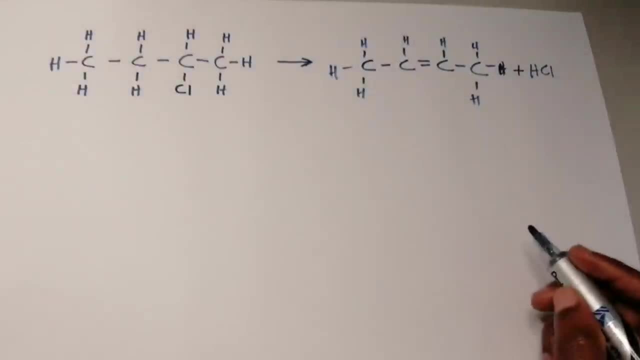 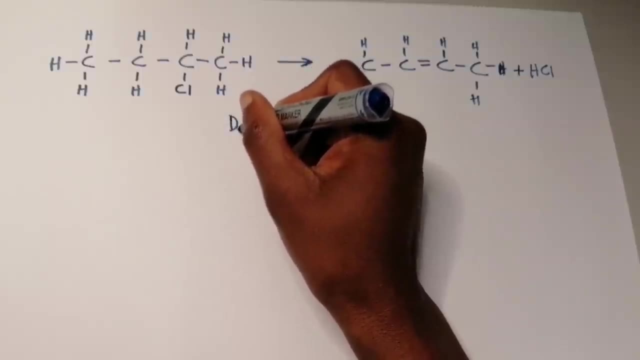 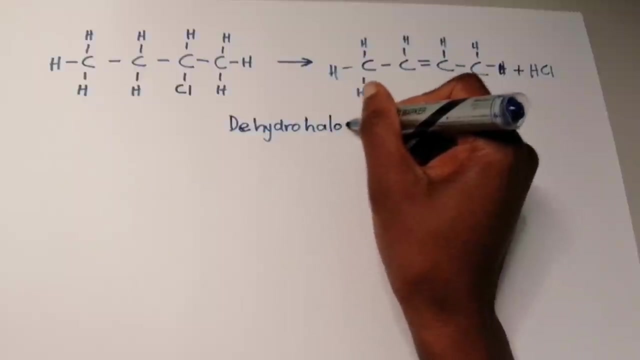 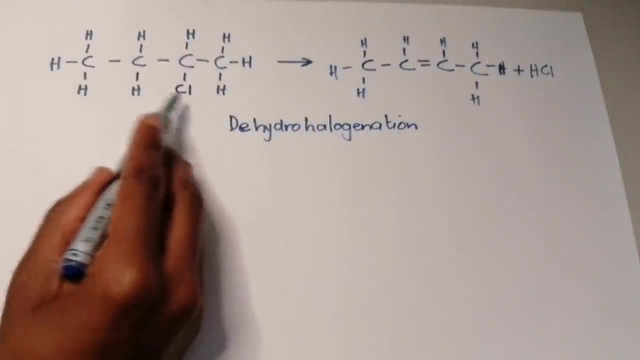 oh, by the way. by the way, sorry, just the name of this reaction. we know it's an elimination reaction, but what type of elimination is it? we call it dehydrohalogenation. this is dehydrohalogenation why? because you remove the hydrogen as well as a halogen as well. 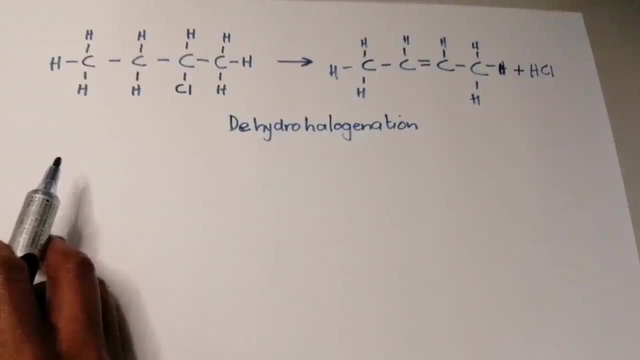 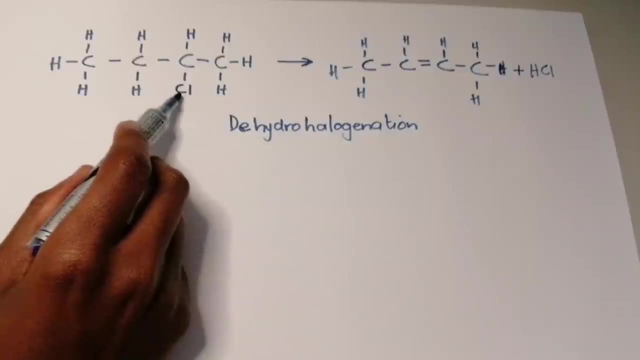 right, yeah, so you can also do this with alcohols. by the way, you would apply the same principle. if you've had an H and an OH there, you can remove that H and OH and that forms H2O on the. 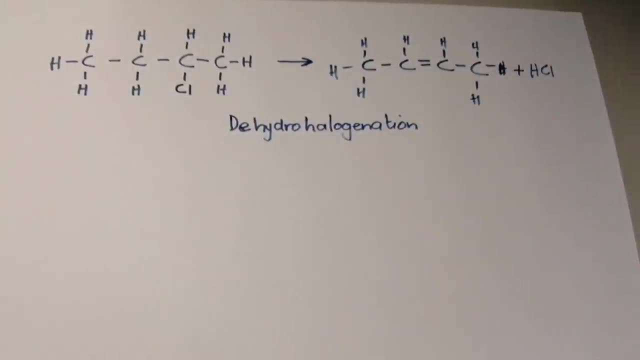 other side. okay, right, so I just want to go through just amongst the last lessons, um, last reactions that I I wanted to show you, right, and then so, um, we're going to take just another reaction, all right, so this is a very popular reaction, uh, that I wanted to explain to. 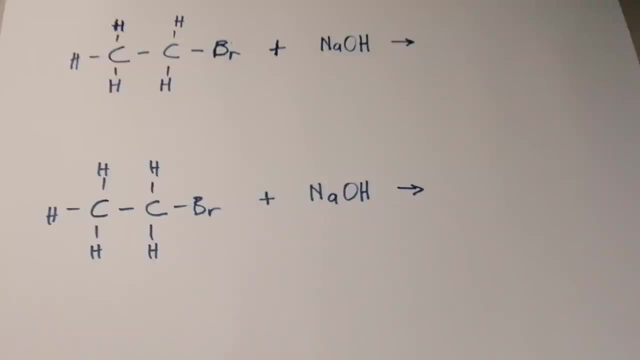 you and take you through. and, by the way, in my previous video, if you want to see the reaction uh for the formation of uh esters, uh, please go to uh the video that I produced before. 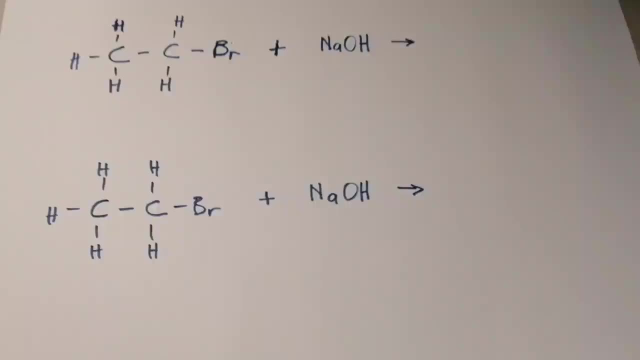 uh on on the naming uh of organic compound. the second video, and you'll see just how to um uh form esters there, right? uh, in case you think I've forgotten about that one, so this is a very popular one, uh, by the way. uh with examiners. 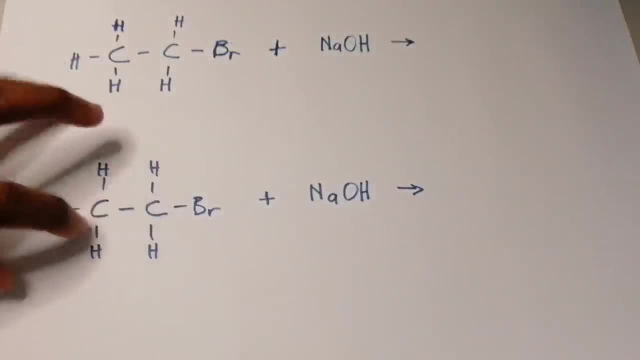 so what they normally do is they would give you either. so when you look at these two reactions, it's exactly the same thing. but what's the difference between the two? it's just the conditions, right? so the conditions of this one. let's start with this one and we say: 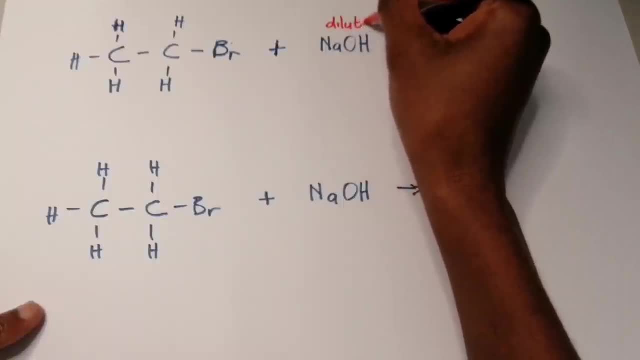 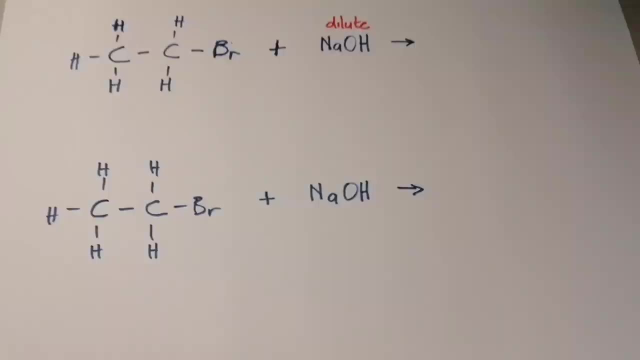 right. what happens when we put dilute um a dilute uh strong base, right? so if I put dilute hydroxide, you can use potassium hydroxide. in that case, right? what type of a reaction occurs? 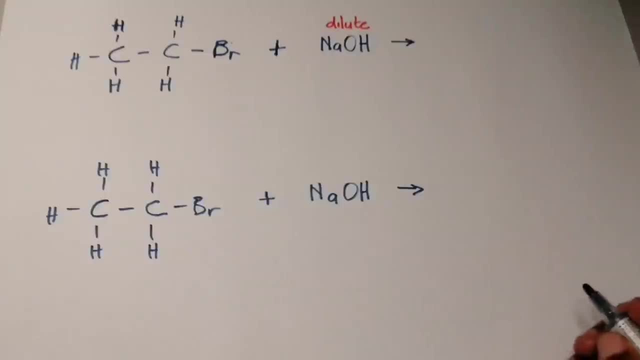 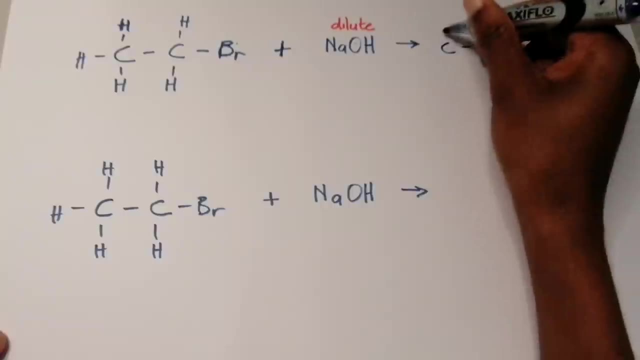 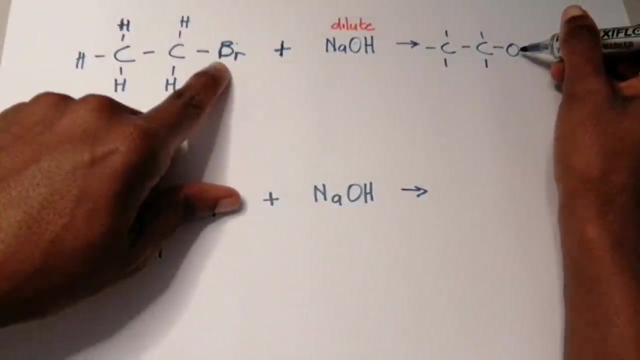 there. note when I, when, when I use a dilute base right, so what I then form is um, an alcohol. so this is another way. so the OH would tend to substitute that halogen there. so I produce an. 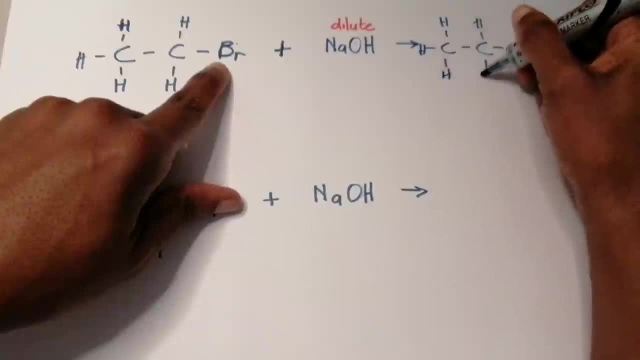 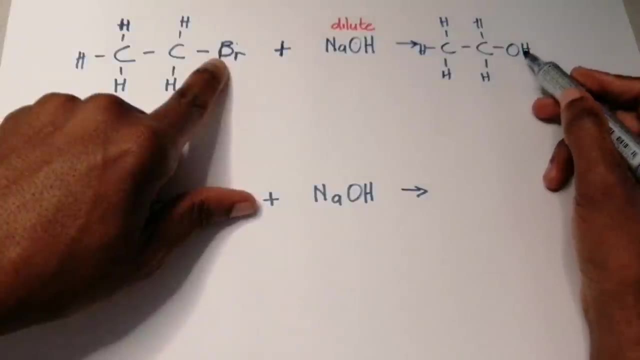 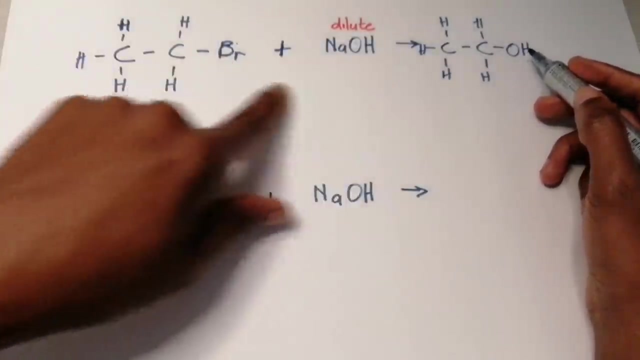 alcohol right. notice what did you uh remove there. you substituted bromide right and um. you substituted OH uh in the place of the bromide ion there. so now you are left with NA and BR. 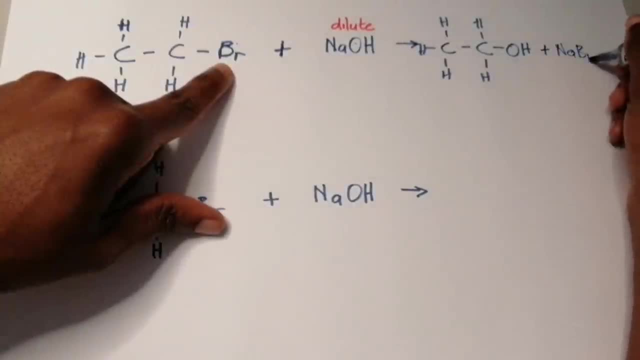 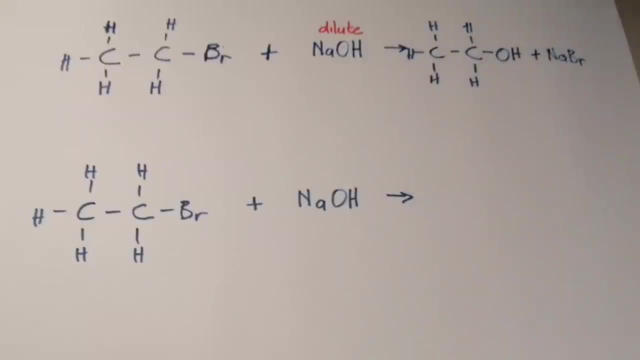 so that's going to be your other product there, right, but in this case it when it comes to organic product, uh, this one is uh formed. Now, please note. the condition there is that our sodium hydroxide is dilute. right, and, but what if I use? 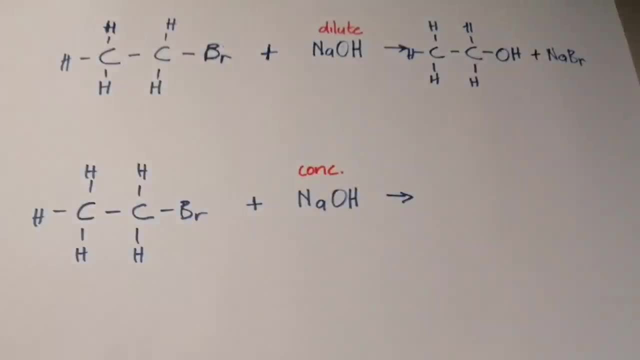 concentrated sodium hydroxide and, by the way, they normally say, uh, at a higher temperature. right so concentrated sodium hydroxide at high temperature. on this one, they would say it in mild heat, right? so now what happens? Instead of an alcohol forming? 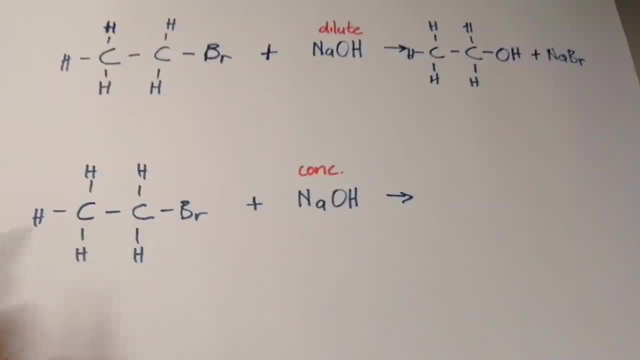 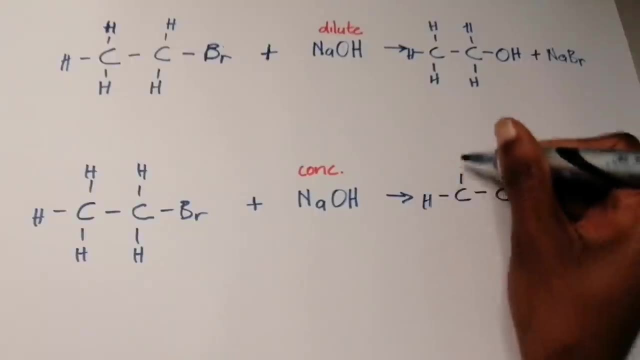 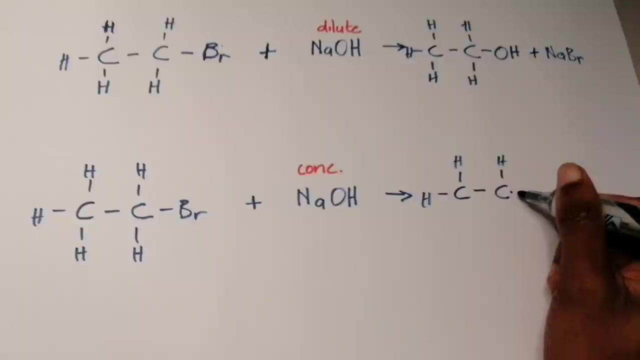 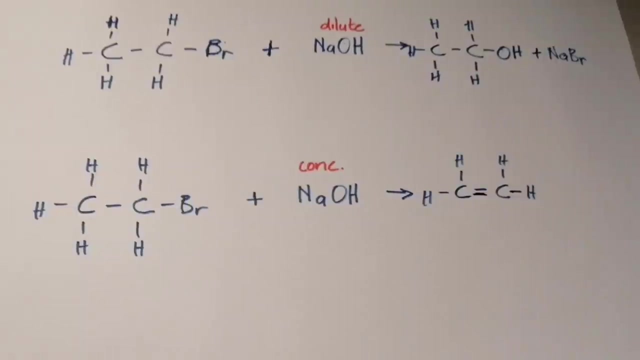 it would be a very dangerous process in this case there, um so yeah, um, euuh uh 물. the second bond, the pi bond, right, So that's an elimination reaction And, by the way, that hydrogen bromide there.